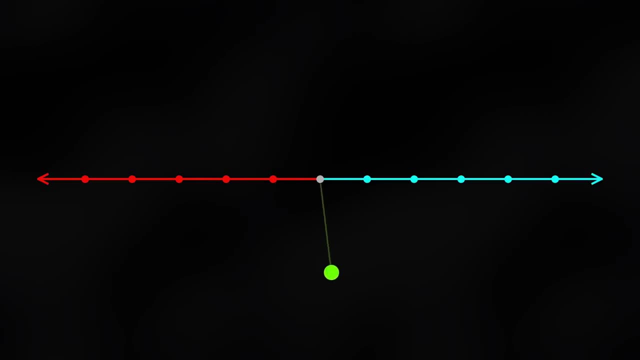 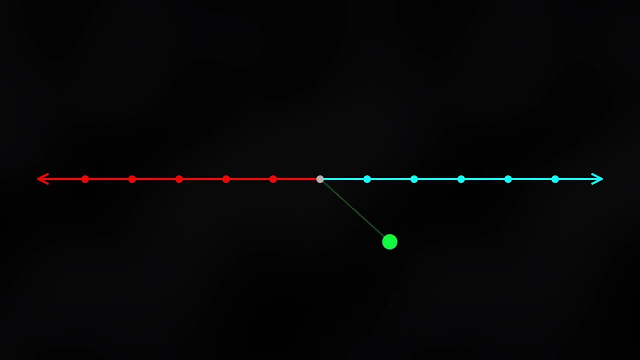 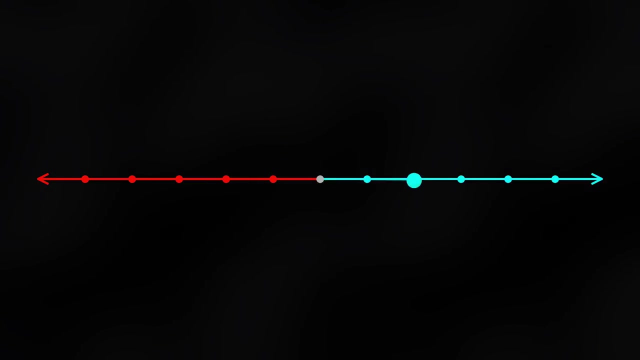 in this space of this, somewhere in this circle that has radius two, The number with magnitude two in the complex plane can be at any one of these points, And that doesn't seem right because, you'll notice, when two is up just purely pointing straight up, then it's neither positive nor 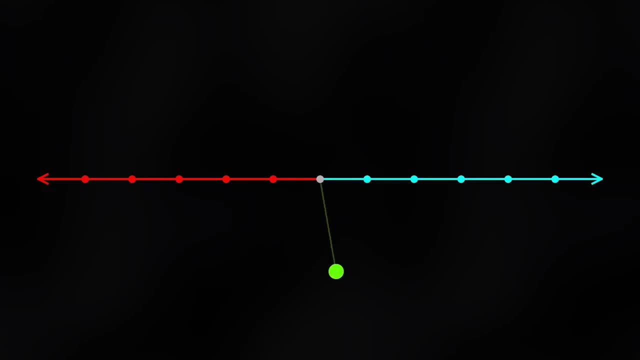 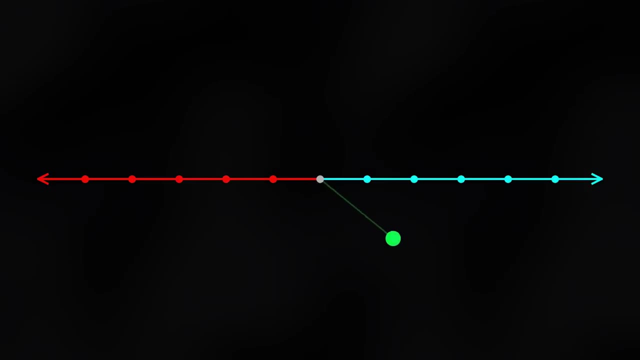 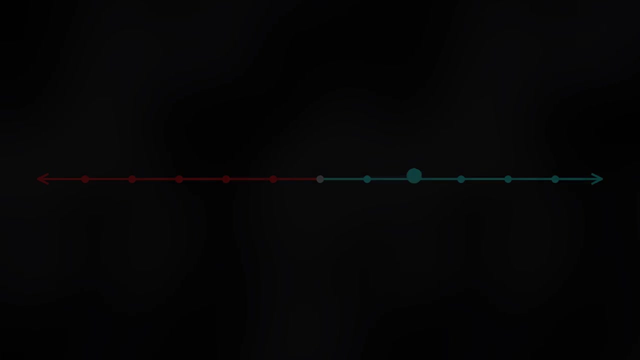 negative And yet it's still two. It still has the amplitude of two. That doesn't really fit into our normal intuitions about counting right. It doesn't feel like it makes sense. Okay, but complex numbers are not about counting in this kind of way. Let's look at this. This is a wave. What kind? 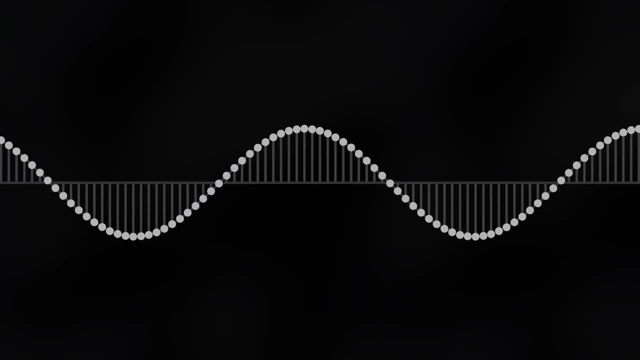 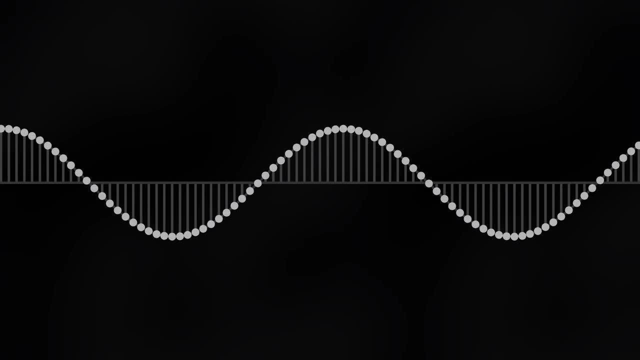 of wave, I don't know. Could be the surface of the ocean. It could be a sound wave, where the height represents the air pressure. It could be a wave of light flopping around in the electromagnetic field. Whatever it is, it's just a wave. Now, this is. 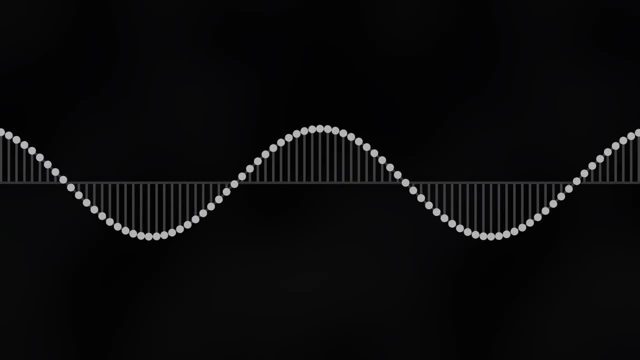 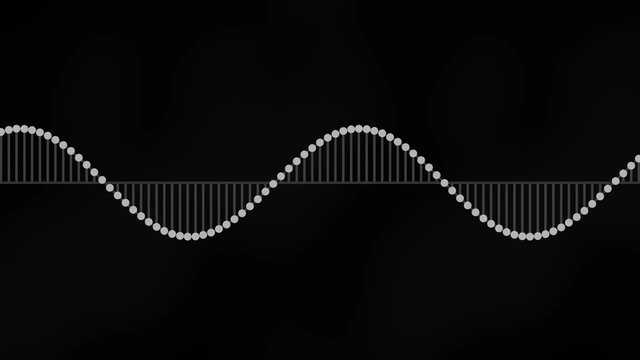 a very clean and pure wave. that I'm using to illustrate the point, but it's a wave nonetheless. So how can we use numbers to capture what this wave is? Well, the first and most obvious thing is: if the wave is above the average level. if the wave is up, we'll say it's a positive number. 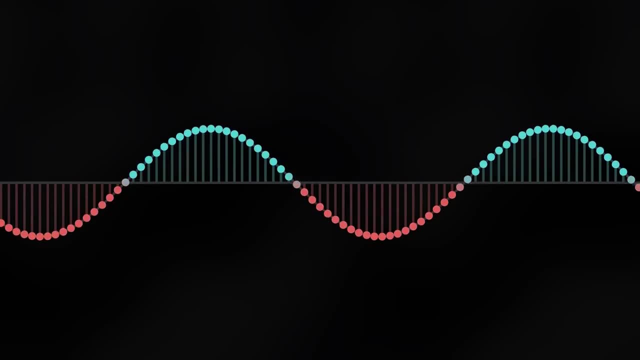 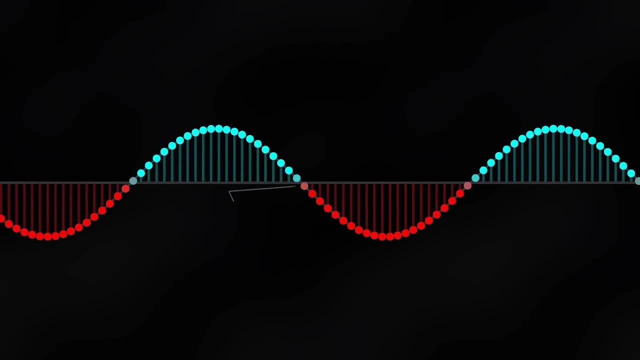 And if the wave is down, we'll say it's a negative number. So let's go ahead and color it in positive and negative. All right, fair enough, It's not wrong. But let's pause time for a second. Now look here, Right at the point where the wave is zero and going down. 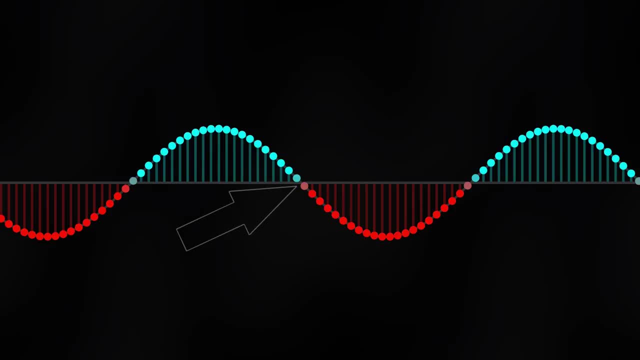 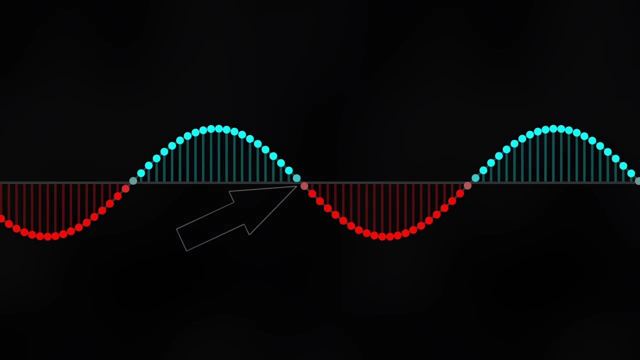 is that point really zero? Or does that point exist in a harmonious continuum with the rest of the wave? Yeah, it's zero now, but it's part of a bigger picture And you know it's just going to be changing soon. You know it'll soon be non-zero. So is that really zero, in the same way that a flat? 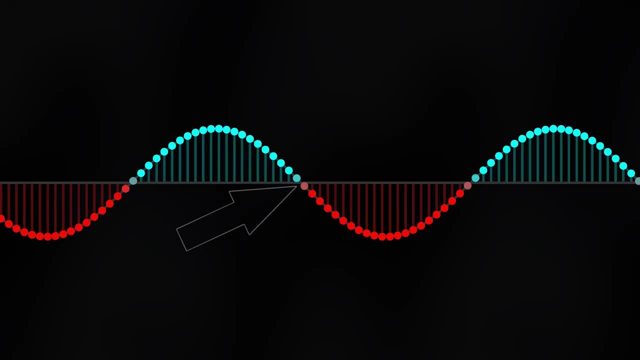 line is zero, Or does it somehow have an amplitude, even though it's also kind of zero at the same time? So do you see an analysis of the wave as being a positive number, Or does it somehow have an amplitude, even though it's also kind of zero at the same time? So do you see an analysis of the wave as? 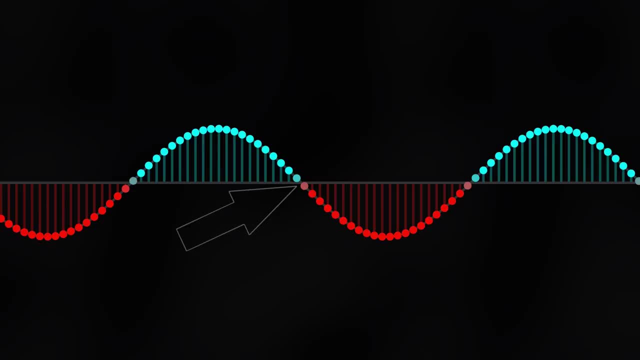 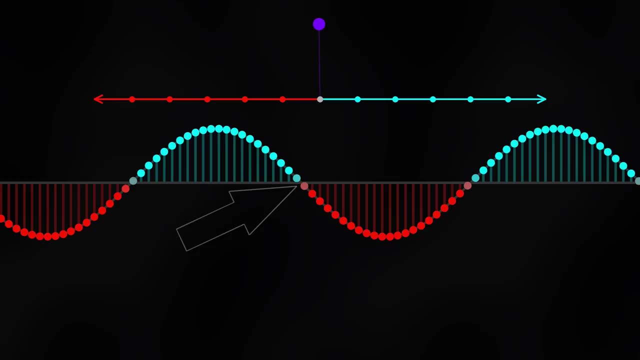 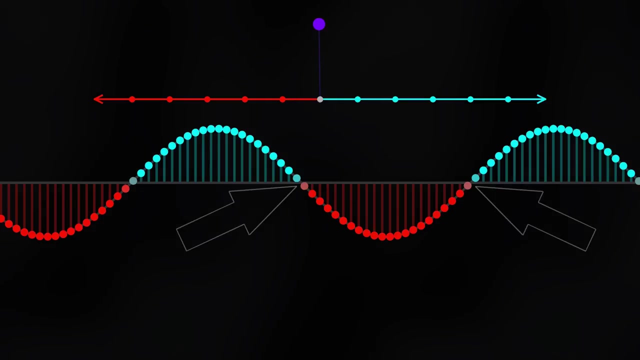 being a positive number, Or does it somehow have an amplitude, even though it's also kind of zero at the same time? here, where it's also zero, but now it's going up, all of the same observations apply: it's kind of zero, but it's not really. it has some energy to it. even though it's zero, it's kind of, is kind of. 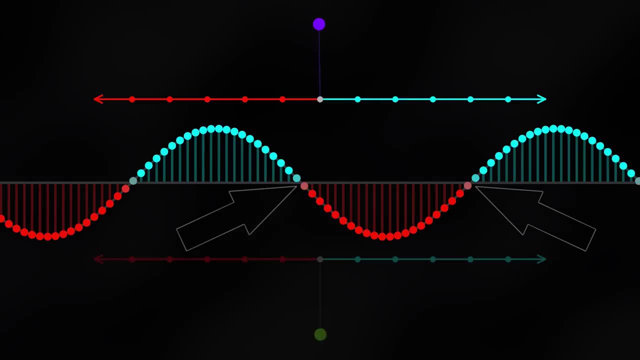 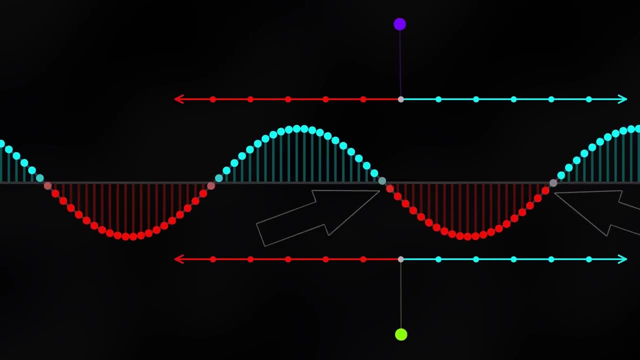 isn't. so now we can see that this number here is the opposite of the previous number that we were looking at, because the previous one is on its way down and this one is on on its way up. Let's transform our perspective and use complex numbers to 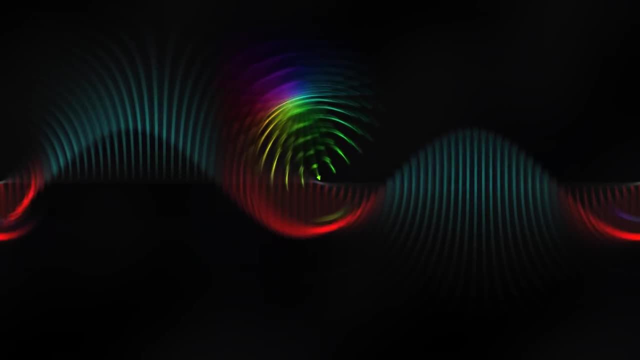 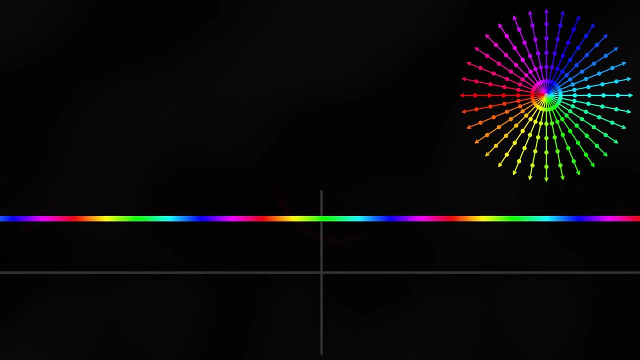 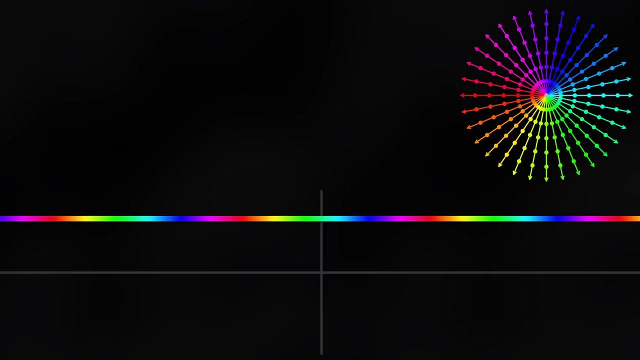 represent this wave. This is what a complex wave looks like. Notice that the amplitude is constant and it's just the phase that's changing, so it's not moving up and down like the other wave. Now, this is a very pure wave. this is a wave of the form e to the i. 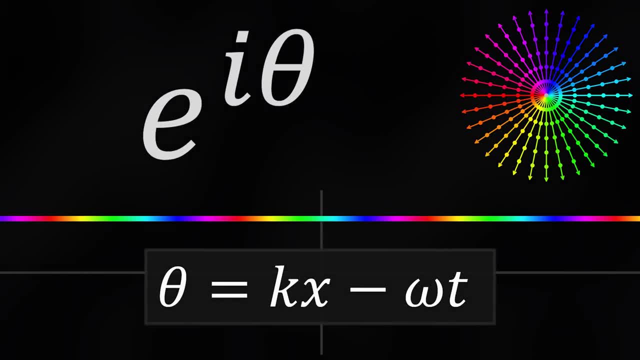 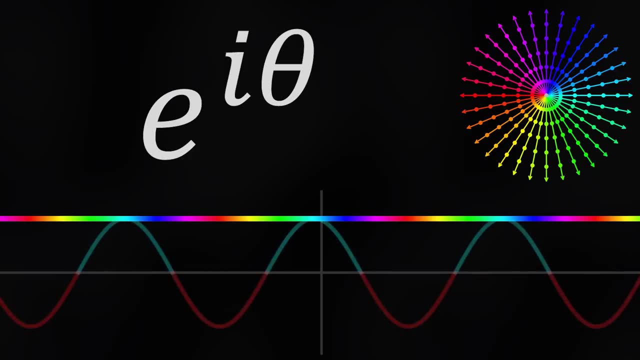 theta, where, in this case, theta is some function of x and some function of time. Now let's plot the real part of this complex number, that is, how far left or right the number is in the complex plane, and you'll see that we can recover that. 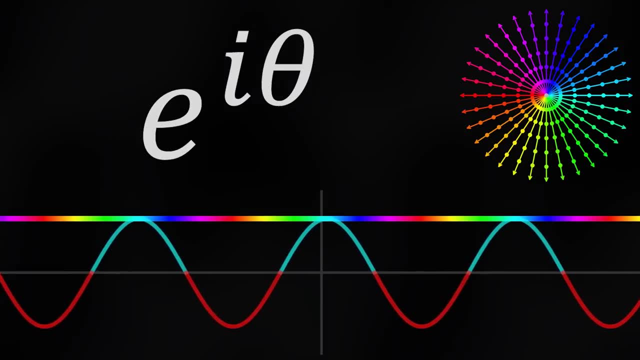 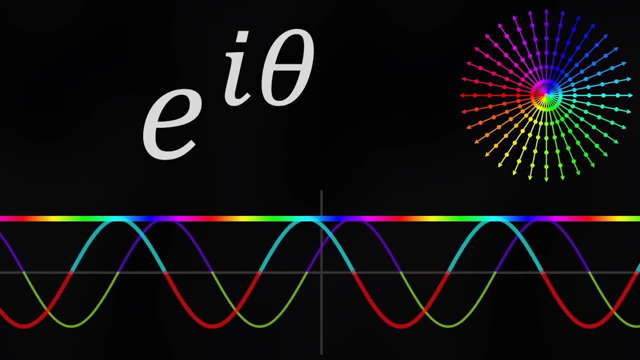 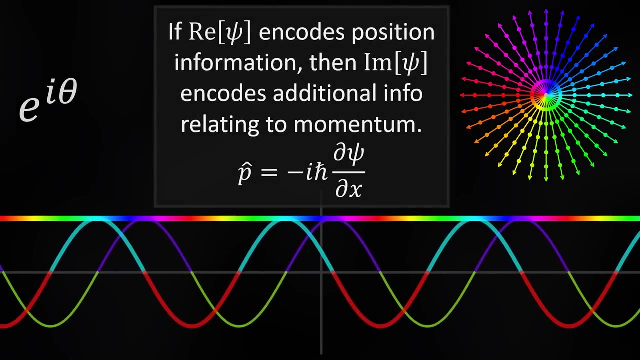 wave we were looking at earlier. Let's show the imaginary component of this complex wave, that is, how far up and down the wave is in the complex plane, and you'll notice. here we get a wave that looks very similar to the real part, but it's out of phase, such that it takes on maximum and minimum values when 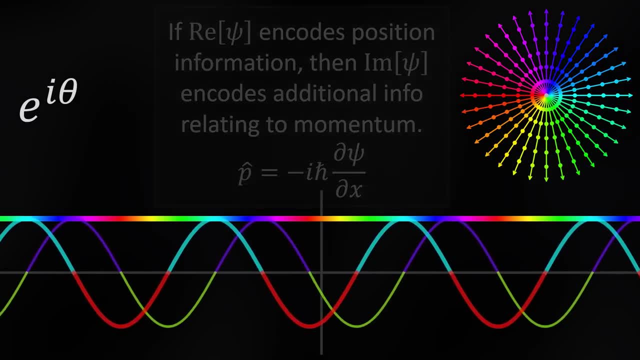 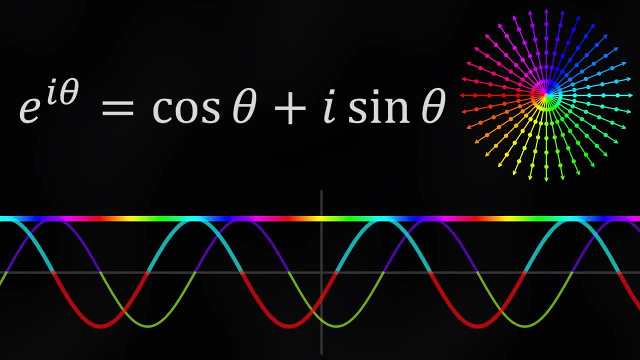 the real part is at zero, and vice versa. By the way, the function e to the i theta is equal to cosine of theta plus i times the sine of theta, where i is the imaginary unit. This equation is known as Euler's formula- well, one of his many. 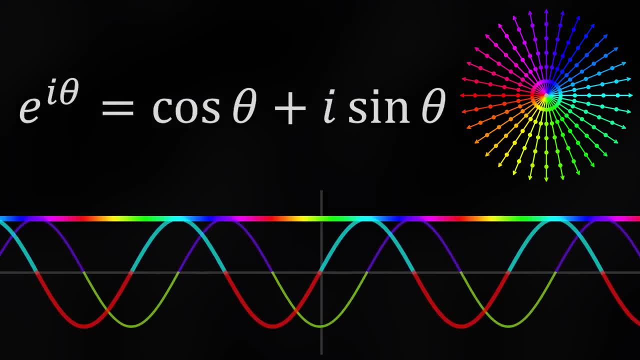 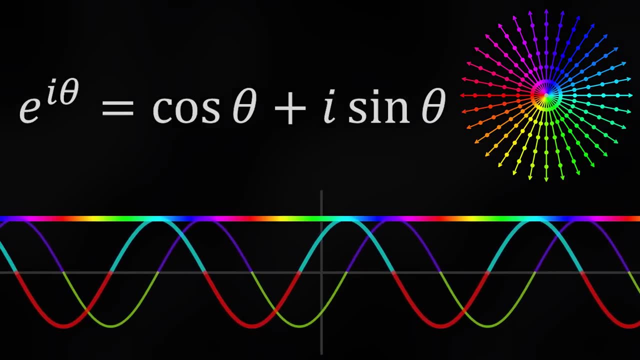 formulas and it gives us another way of thinking about what this complex wave is. When you're first getting into complex numbers, you will probably think about Euler's formula as the definition of what e to the i theta is. but as you become more comfortable with e to the i, 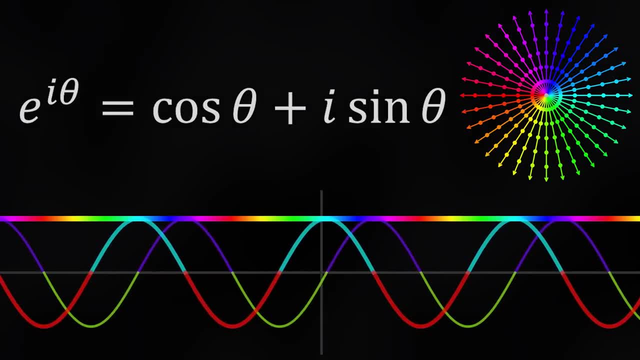 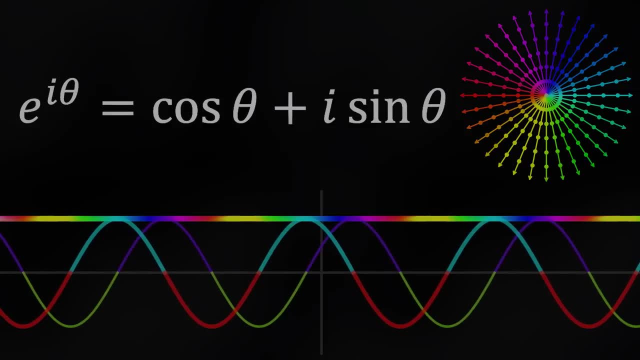 theta. you'll eventually just see that as the wave and then the cosine and sine as a way of splitting it up into the real parts and the imaginary part. By the way, let me just quickly say on the topic of the imaginary part, imaginary numbers. 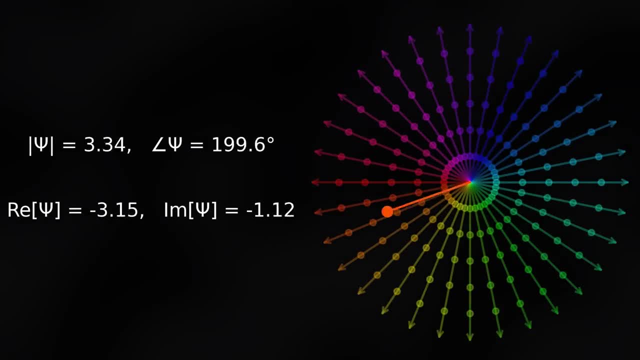 are a misnomer. okay, They're just as real or just as imaginary as the real numbers. The complex numbers are a numerical structure. they're a holistic thing. you know. it doesn't make any sense to say imaginary and real. 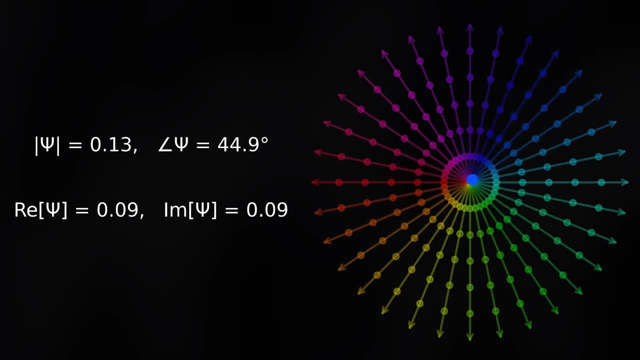 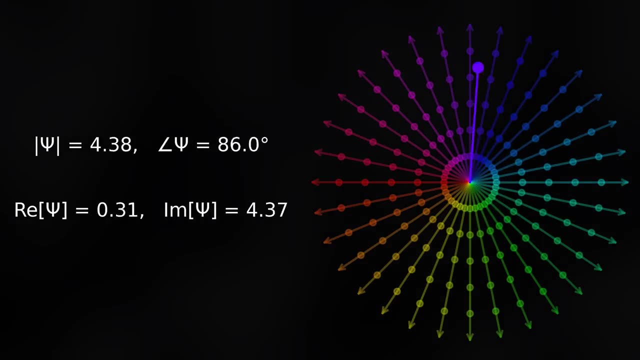 but whatever, this is the terminology we're stuck with, so it is what it is. Ultimately, it's a consequence of the fact that the imaginary numbers were named before they were understood, and that's, I think, one of Descartes's greatest mistakes. Well, that, and dualism. 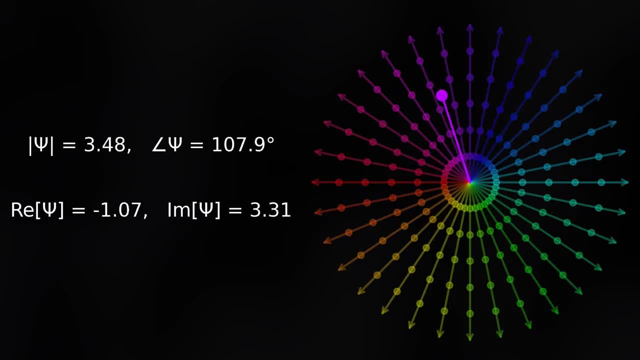 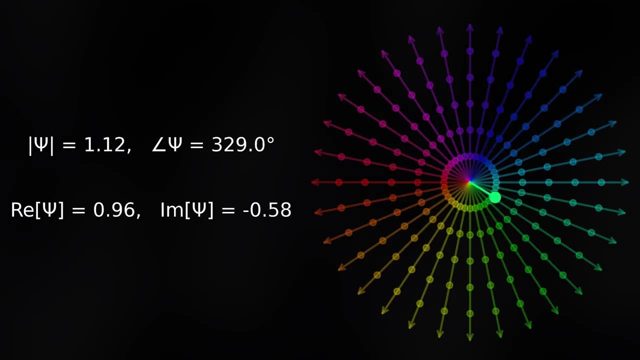 but um, Anyway, where were we? What are we talking about here? To understand why it's useful to be able to represent a wave as a constant-amplitude, complex number whose phase is changing, we'll have to take a look at the nature of complex addition, multiplication and how this relates to wave interference. 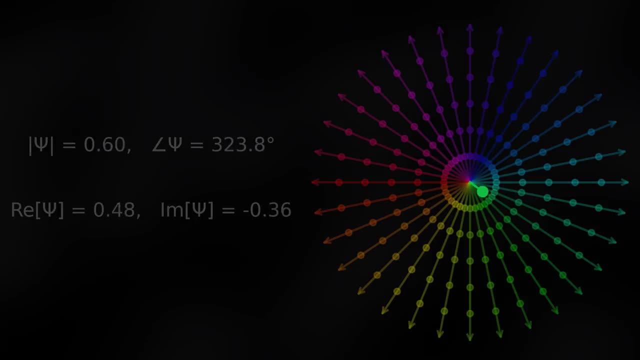 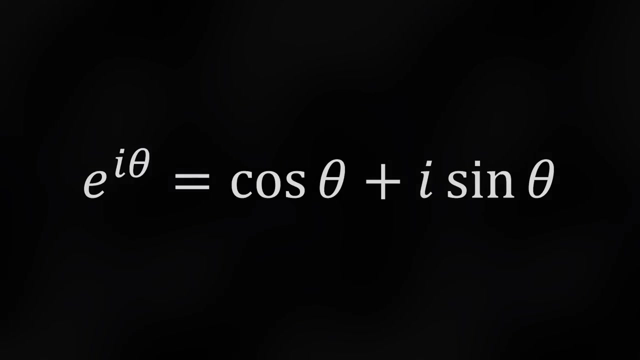 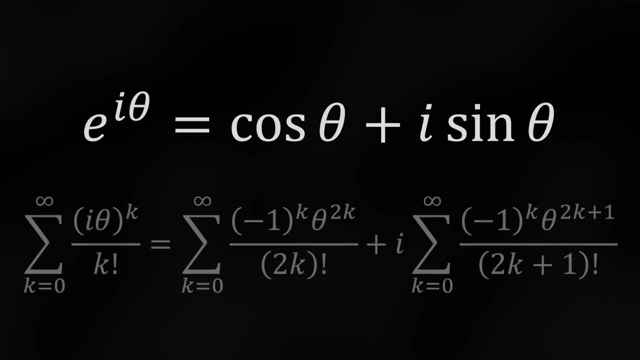 interference. We'll do that in a moment, but first I want to make a quick comment about why is it e to the i theta gives us this wave? I don't have time in this video to give a really satisfactory answer, but I can lead you in the right direction. So if you take derivatives of e to the i theta and 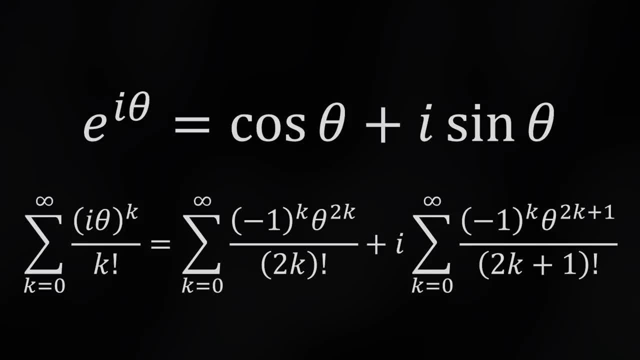 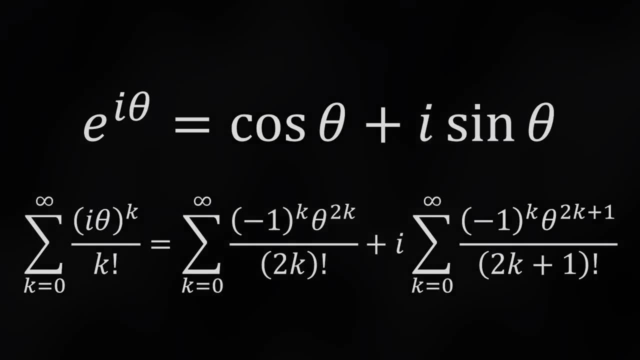 sine of theta and cosine of theta. you can write these functions in terms of a Taylor series. When you do that, you'll find that e to the i, theta has a term of theta at every degree, whereas cosine has even terms and sine has odd terms. And if you look closely at these series, 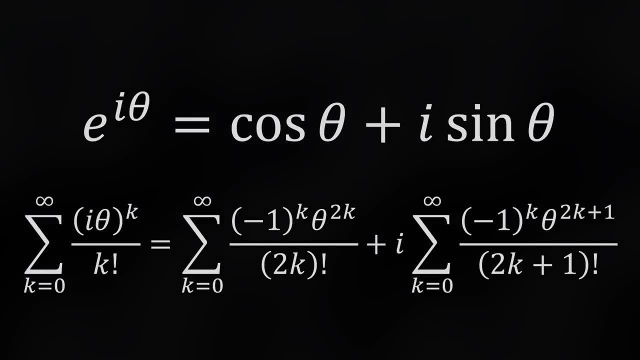 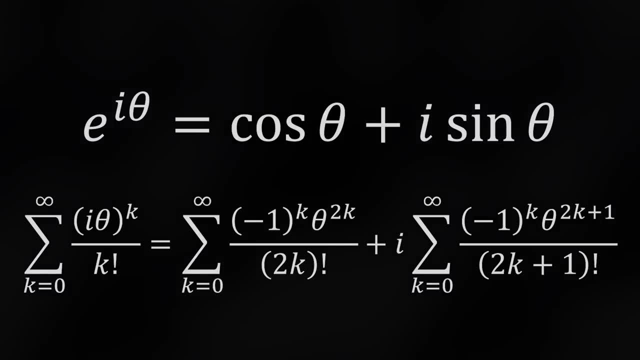 you can see that the terms on the right hand side of the equation zip together into the terms on the left hand side of the equation. So by taking Taylor series you can prove to yourself that in fact, e to the i theta is cosine of theta, plus i sine of theta. Okay, so that was a bit of a. 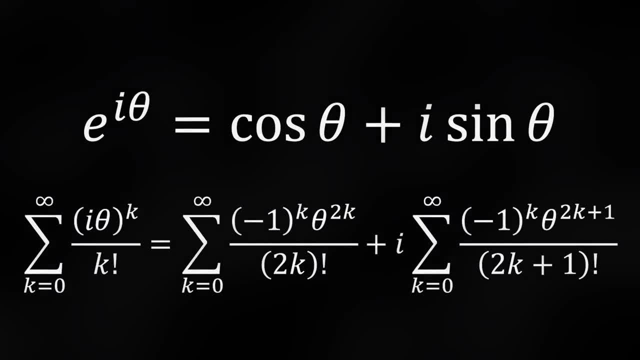 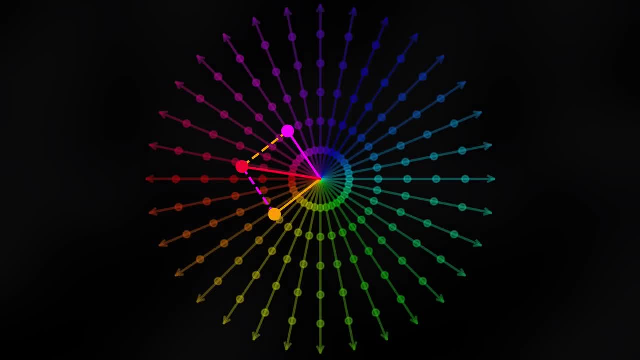 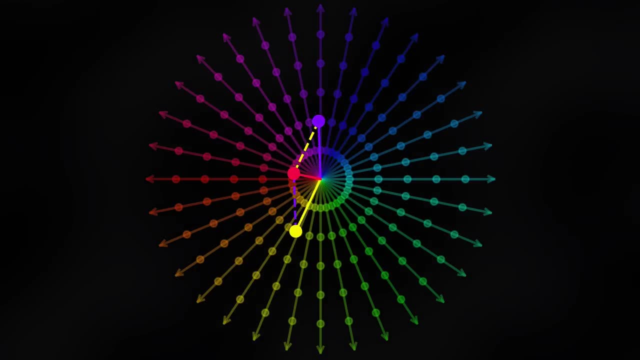 tangent, but I think it's important for you to know. Now let's take a look at complex addition. If we have any two complex numbers, we can add them, just like they're vectors. So we put them tail to tip, or another way of looking at it is: the sum is the diagonal of the parallelogram. 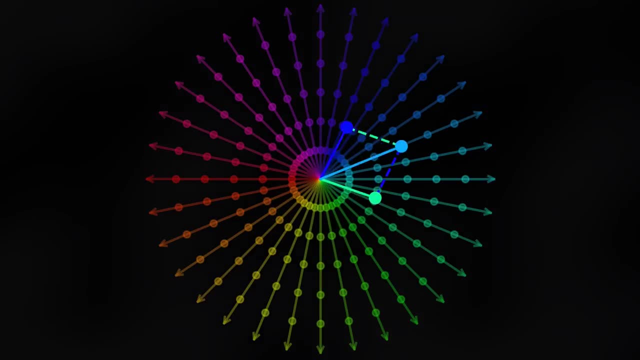 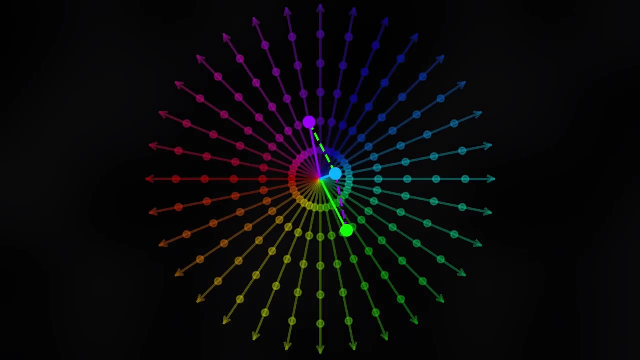 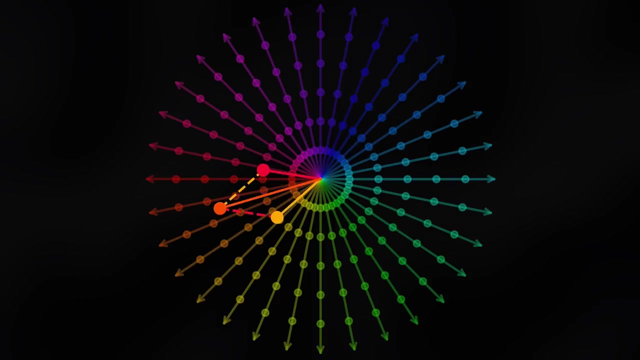 So here I'm showing two complex numbers, both of which have magnitude two, swinging around in the complex plane. The complex number between them is their sum, And you'll see that, since the numbers both have magnitude two, their sum has a magnitude of anywhere from zero to four, Zero when the two 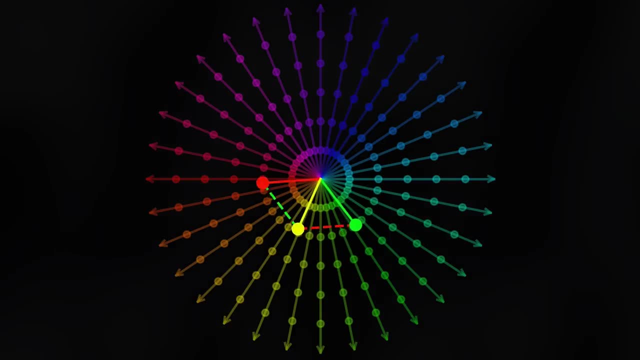 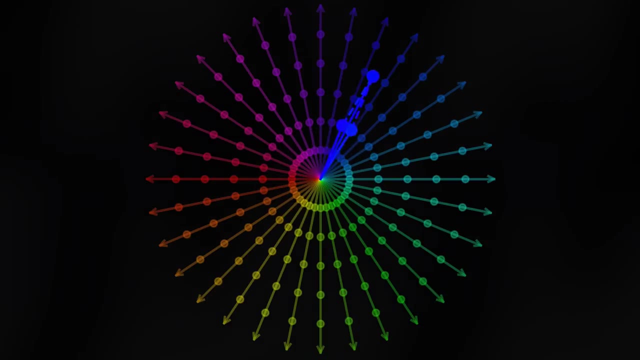 are perfectly out of phase four, when the numbers are perfectly in phase and some intermediary value, when the angles are kind of in phase and kind of not in phase, And we'll see later how that has a very close relationship to the idea of constructive and destructive interference in waves. 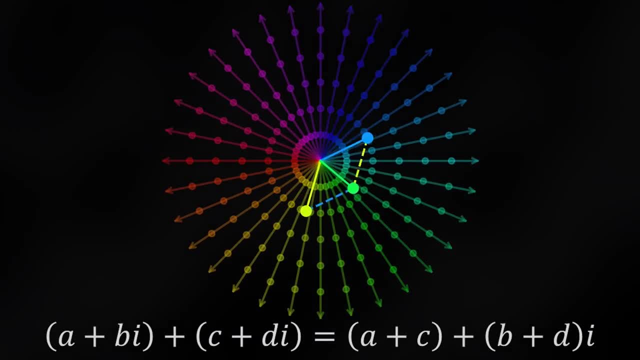 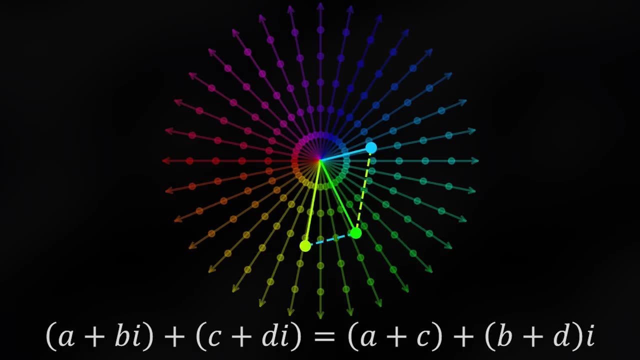 By the way, here's the algebraic formula for complex addition, and that's the same as adding vectors, like the animation shows. Now let's let one of those two become a little bit longer And you can see a more general representation of complex addition. And you still see this effect where sometimes the numbers 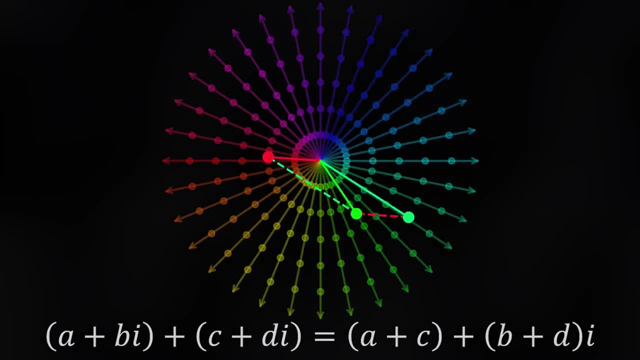 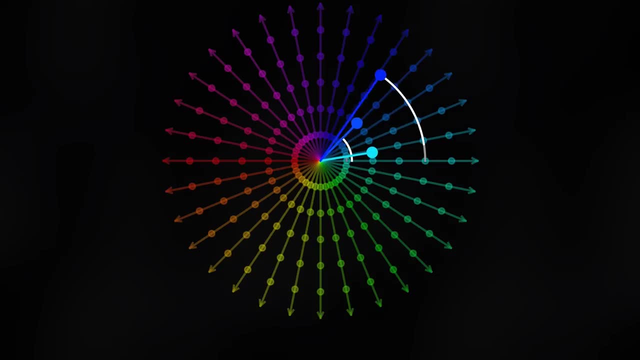 will align with each other and will add to the magnitude. sometimes they'll be oppositely aligned and they'll sort of destructively interfere. So that's a general phenomenon whenever you're adding complex numbers, And we can also multiply any two complex numbers. So to multiply complex numbers, you multiply. 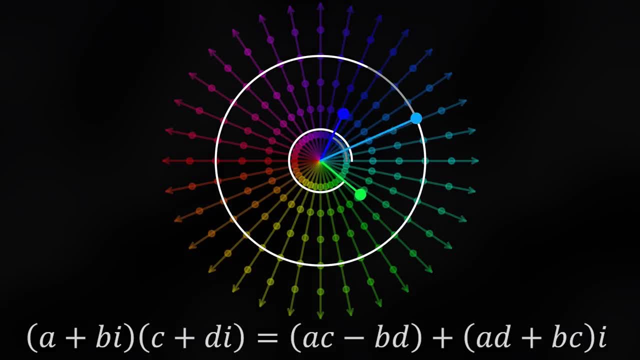 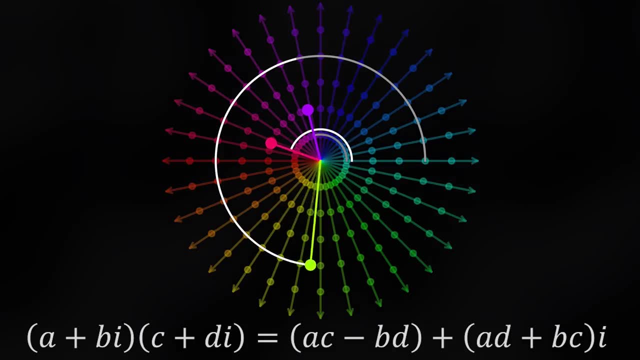 their amplitudes and you add their phase angles relative to the positive real number line. So here I'm showing a couple numbers, both with magnitude 2, they're swinging around in the complex plane, and I'm also showing their product. You'll notice that since the two numbers both have magnitude 2, their product will. 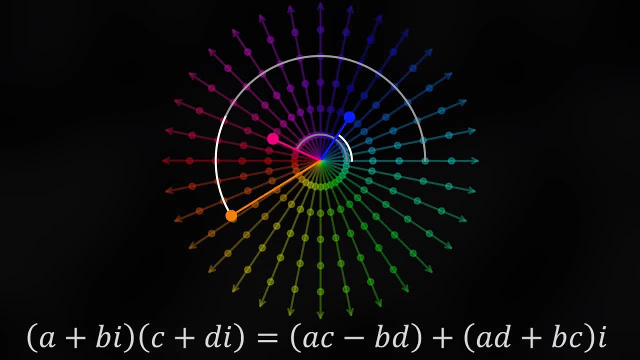 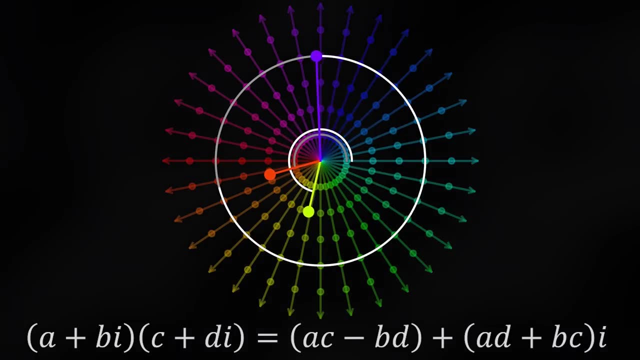 always have magnitude 4, but the phase angle of their product depends on the sum of the phase angles of the individual twos And of course that rule generalizes So any two complex numbers. to multiply them, you multiply their magnitudes and add their phase angles. That's really useful, because what it 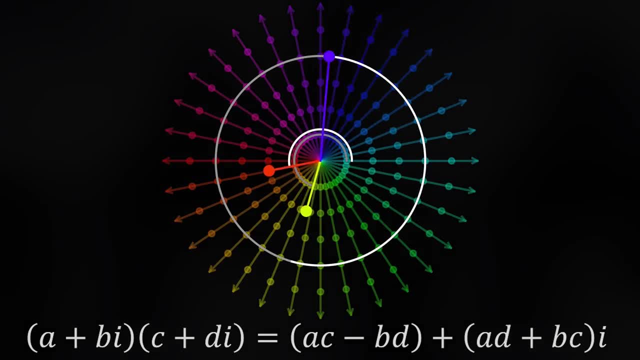 means is that if we have a complex number of unit length but some phase angle in the plane, then we have a phase angle of unit length. So if we have a complex number of unit length but some phase angle in the plane, we can multiply. 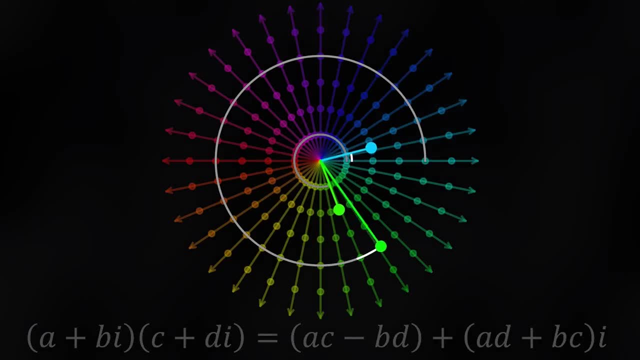 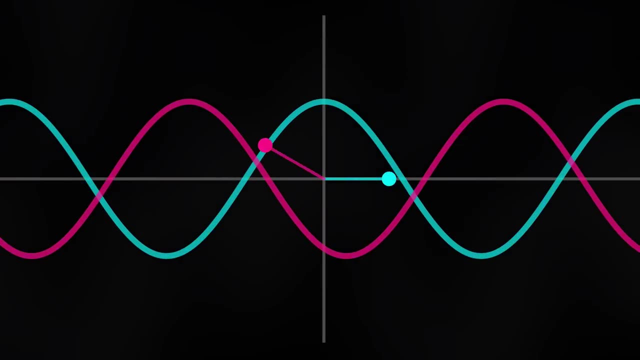 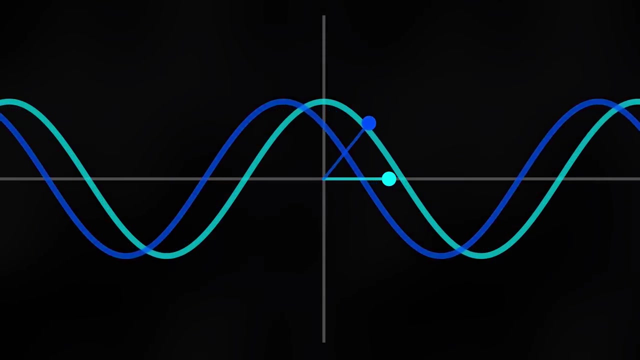 that by some other complex number to shift its phase by the unit one number's phase angle. To demonstrate this idea of rotating the phase of a complex number by multiplying by a unit length complex number, consider the illustration that's on your screen now. Here I have a blue wave and that's the real part of the 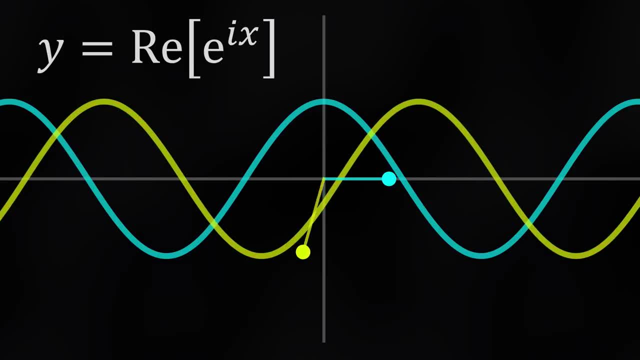 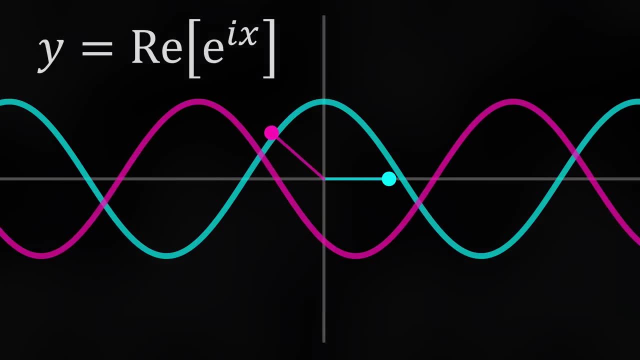 function e to the ix. So the classic complex wave amplitude. one function. you take the real part and it's basically it's just cosine of x right Now, the way that's changing colors. that's the same function, That's the real part of the same. 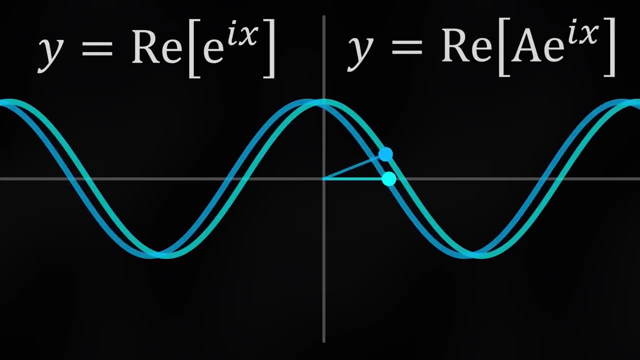 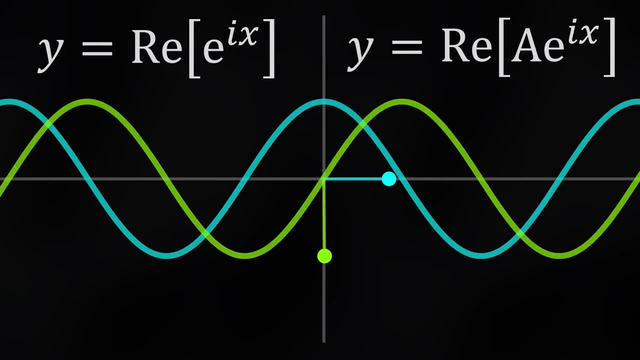 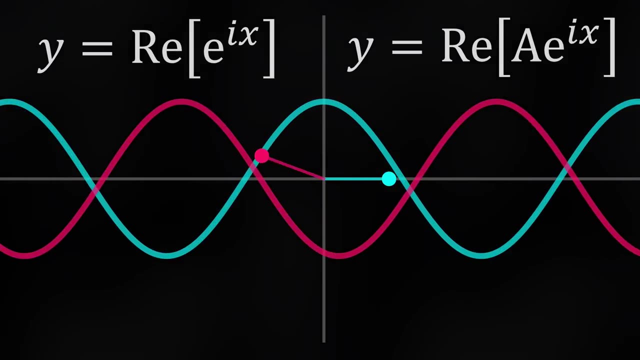 function. except now the function is multiplied by some complex constant. Let's call it a. A has magnitude one, but its phase angle is changing. So I'm showing you here the blue line with the dot at the end. That's the number one in the complex plane. right, The colorful line with 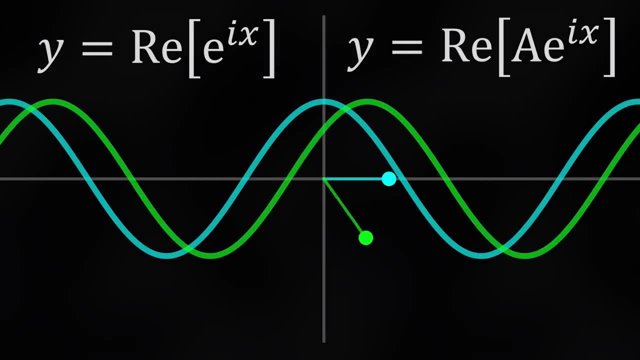 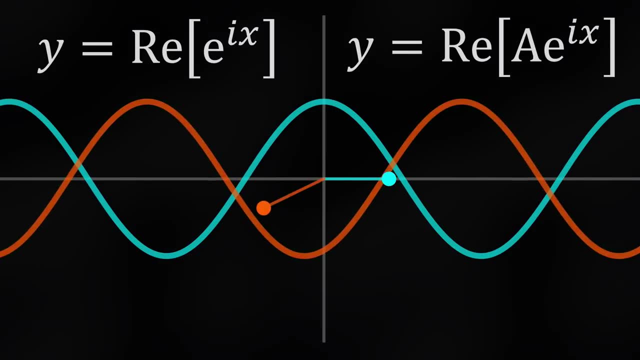 the dot at the end. that's a. That's this unit length, complex number whose phase is swinging around, And the colorful wave that's changing colors. that's the number one. So that's the real part of the wave that you get when you multiply by the complex number a. Now let's 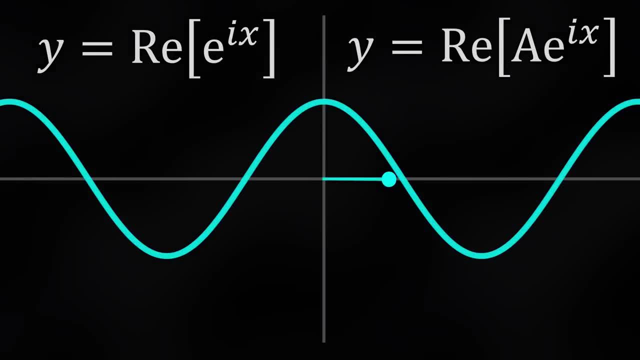 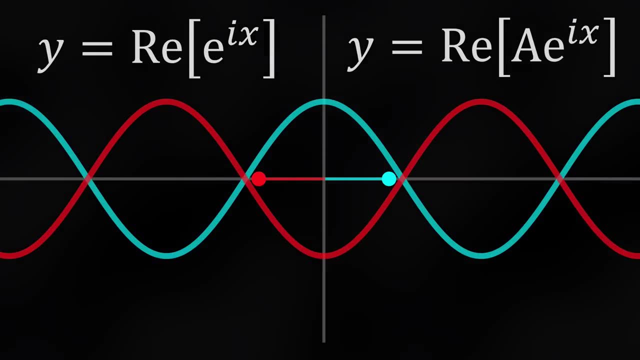 notice something: When a is one, the two numbers overlap and the two waves are the same. When a is negative one, the two waves are completely opposite. So the sign of the wave is switching at every moment. What was formerly up is now down, and so on. But in all those angles, in 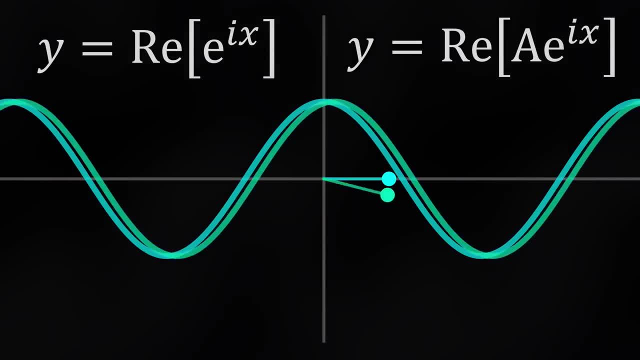 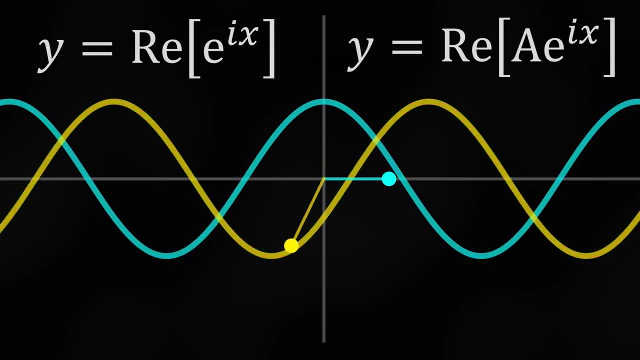 between the waves are not just the same or not just totally opposite, but they're similar. They're phase shifted by some amount- That's not a complete half wavelength, And so in this illustration you can see how this notion of generalizing positivity and negativity that we see in the complex numbers actually 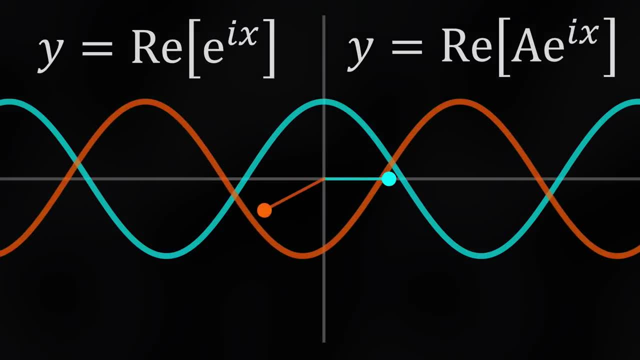 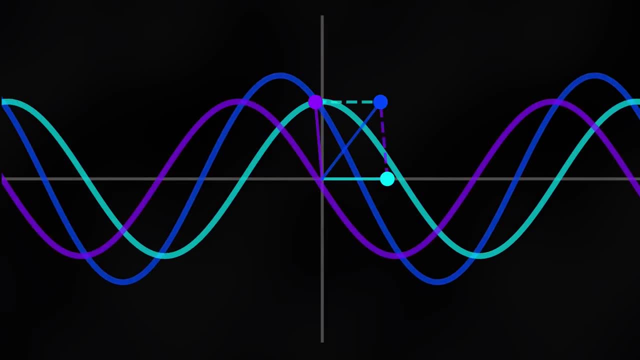 has a genuine, natural, very real interpretation. We can see this even more clearly if we put the sum of the two waves into this illustration as well. Now we can think about addition of waves in two ways. First, you can sweep along the x axis and just add the value of the two. 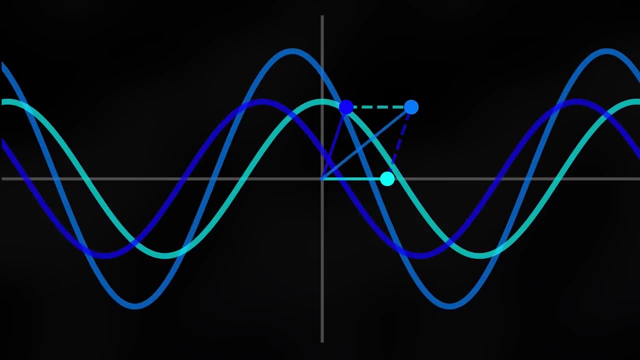 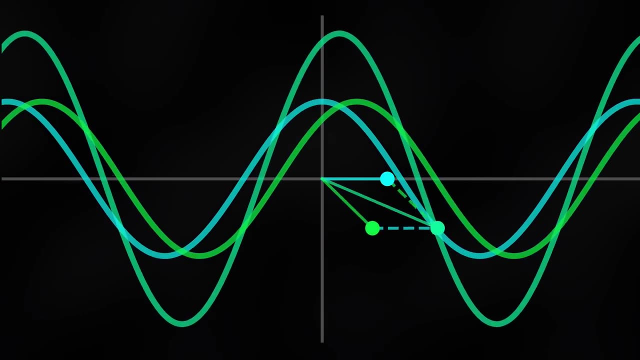 waves at any point And that gives you the value of the third wave. And to do that you can go to the complex amplitudes of the waves. You get a resulting complex number That's the sum of those complex numbers, And then you multiply that by the. 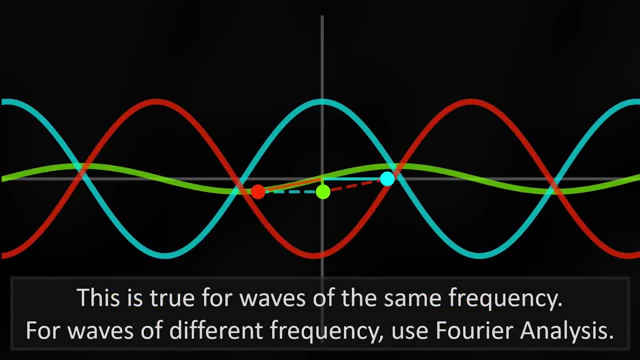 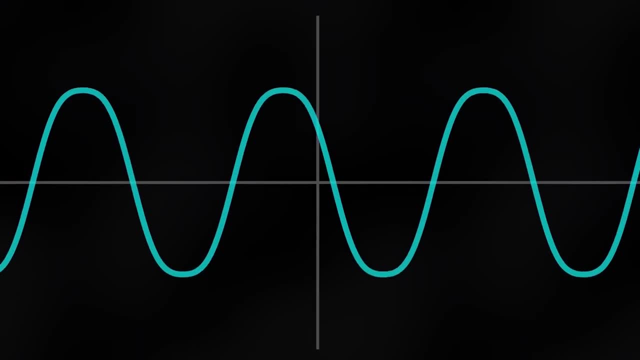 wave e to the x and that gives you the sum of the two waves. So you see, there's this direct one to one relationship between complex addition and the interference of these waves. If you've studied signal processing then you know that you can generate an arbitrary. 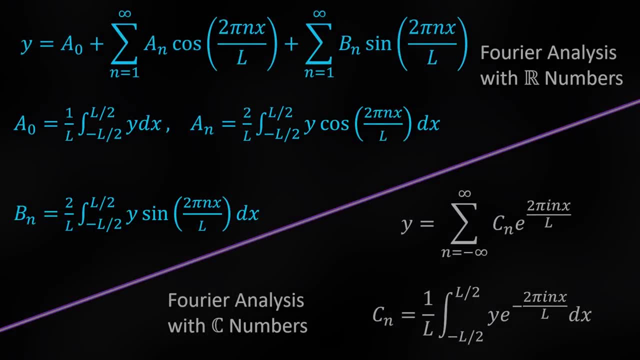 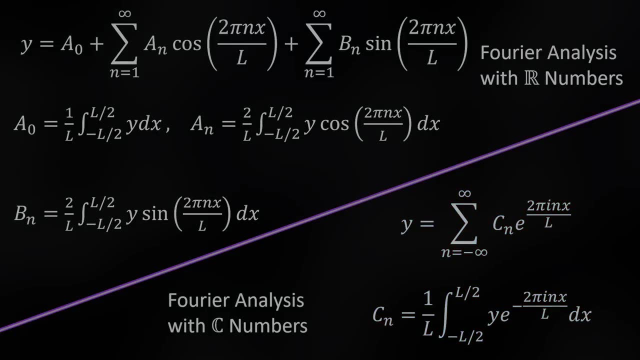 waveform by adding sine waves and cosine waves in the right amounts and frequencies. Well, let us create a more unified and holistic way of doing. Fourier analysis by adding waveforms that are these e to the i, x kind of waves multiplied by a complex coefficient, and then summing over 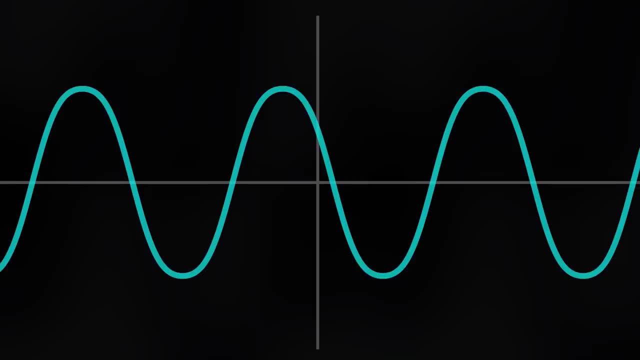 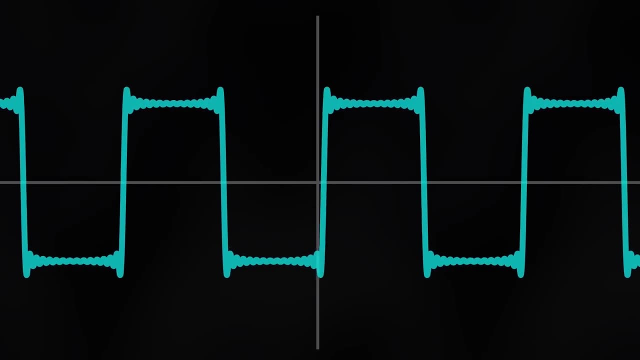 frequencies and amplitudes in that basis. So the example I'm showing here of generating a square wave, you might associate that more with like signal processing or something In quantum mechanics. however, we use the idea of basis functions and superpositions all the time. Consider, for example: 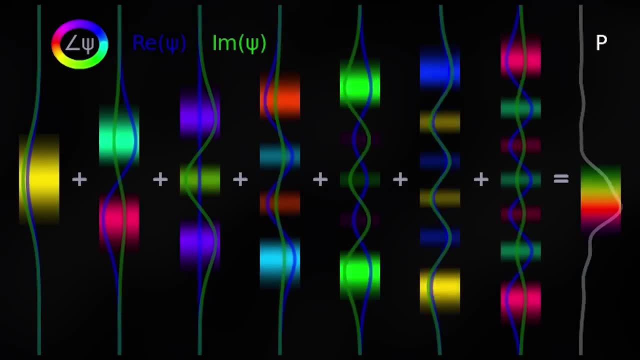 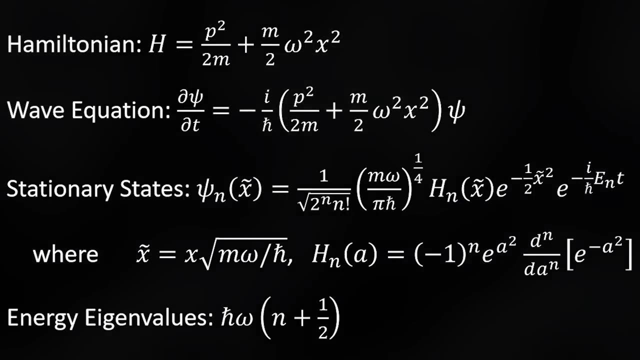 the quantum harmonic oscillator. I already made a video on the quantum harmonic oscillator so I'm not going to rehash all of the details here. If you want to see, like the Hamiltonian and Schrodinger's equation and all that good stuff, you can check out that video. but what I just want to point out here, 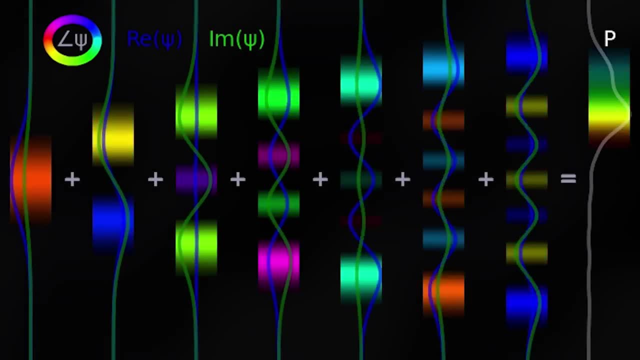 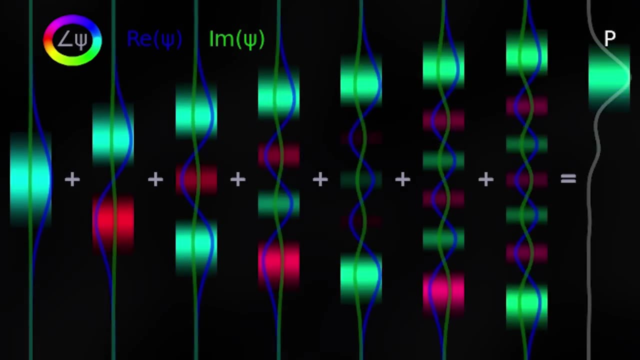 is that we can take this sum of energy eigenfunctions, the ground state and these few excited states and if we add them all up, we can get the wave function of a particle that's oscillating in the quantum harmonic oscillator. And this is just one of the many ways that these 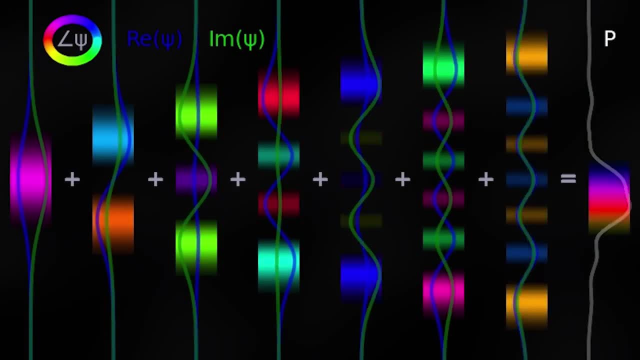 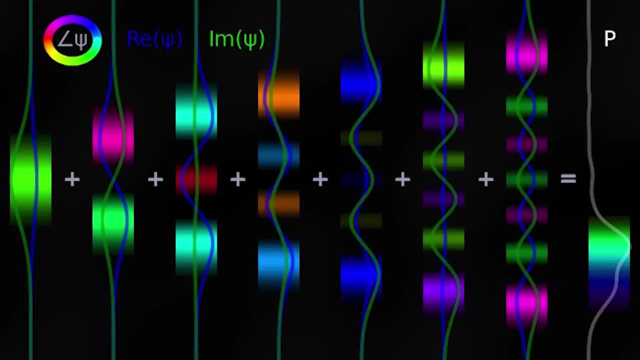 basis functions can be added. But when you look at it, one thing to notice is that if you just look at the probability densities of each of the energy eigenstates, they're actually stationary. But when you add the eigenstates, because you're adding the complex numbers and there's that complex interference- 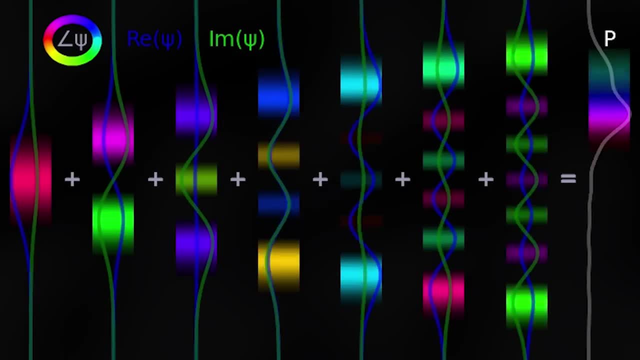 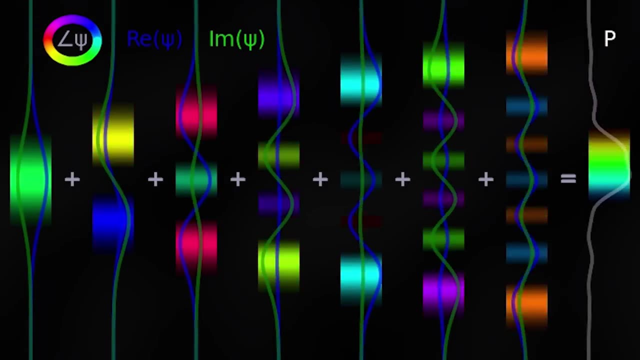 going on. the subsequent probability density of the sum of those states, the superposition of those states, is actually this thing that varies in time, And so here we can see this cool kind of dynamics coming out of the machinery of complex numbers. My main point in this video. 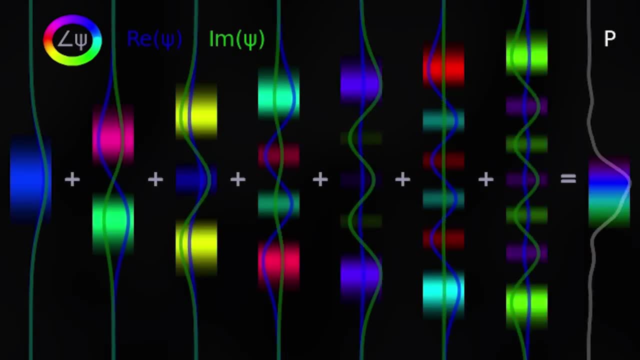 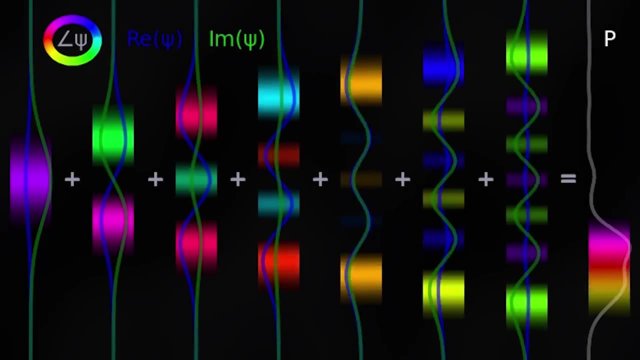 is just to get you familiar with the complex numbers, to show you that ultimately they come from this notion of waves, and we'll see many examples of complex wave functions going forward. For example, I'm currently working on a video on the hydrogen atom, and so here I'll show. 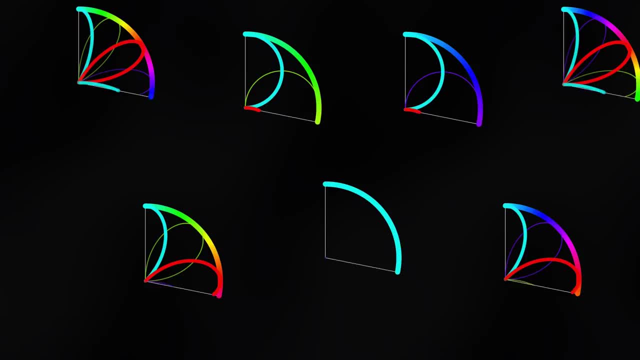 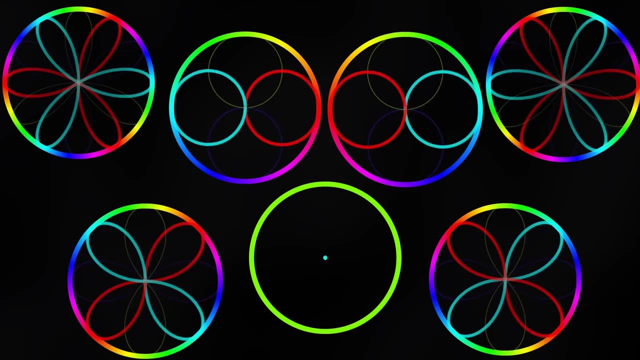 you just a little preview of that. We have the longitudinal component of the hydrogen energy eigenstates. So this is what you get when you solve the azimuthal equation. You end up with the Hemholtz differential equation and you can derive the fact that hydrogen 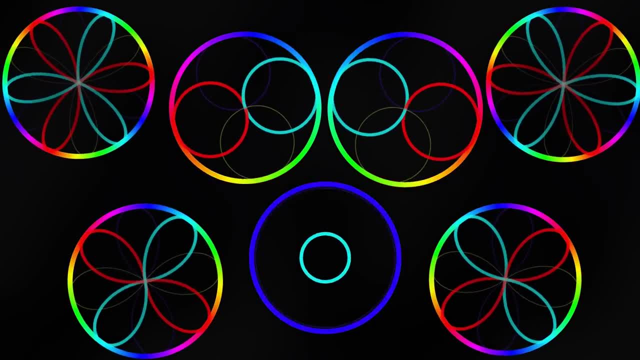 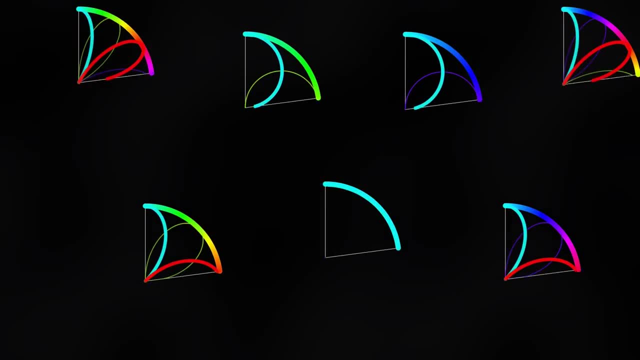 has this quantized magnetic number m, which we learned about in physics, And you can derive the chemistry from the fact that the wave function has to loop back in on itself as you go around. Anyway, we'll come back to this later in the hydrogen video, but for 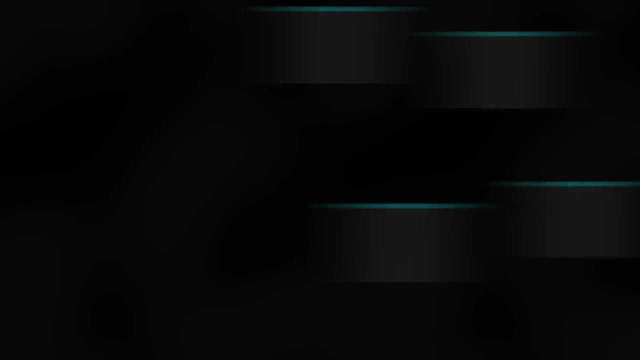 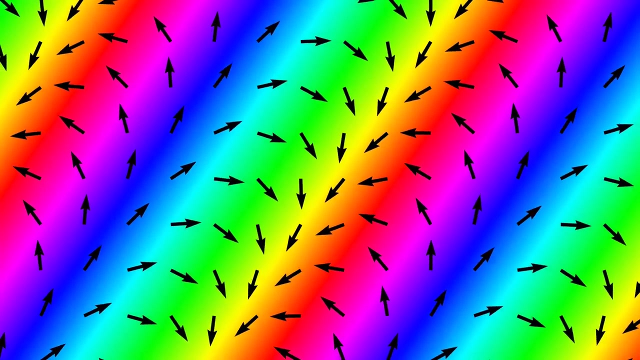 now I'd like to look at a higher dimensional example of a complex wave function. So, for example, here's a two-dimensional plane wave. It's defined in the plane of your screen. its constant amplitude and the color represents the phase of the wave function at every point. 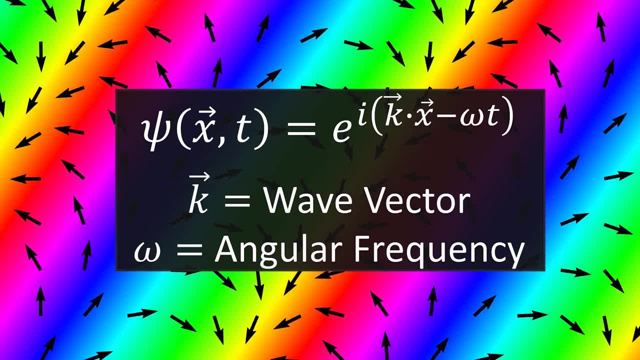 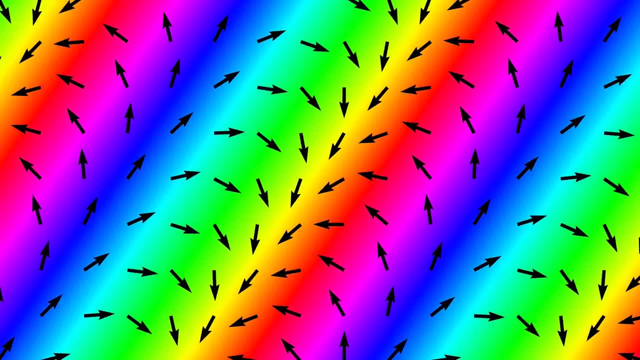 I've also superimposed these little arrows, and what the arrows represent is numbers in two dimensions. Now I want to use this to illustrate a couple of points. First, when you look at a picture like this, it almost looks like a vector field and there's a temptation. 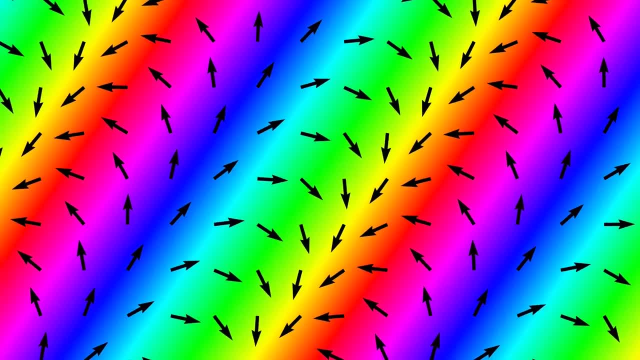 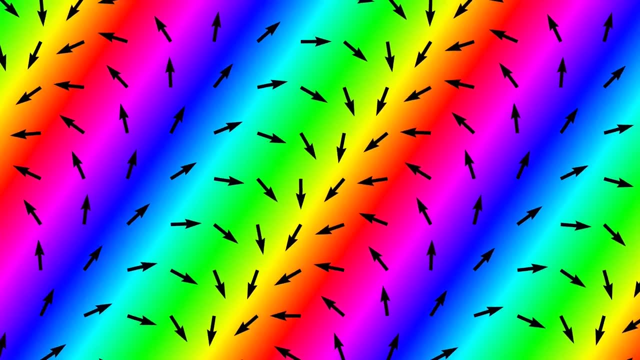 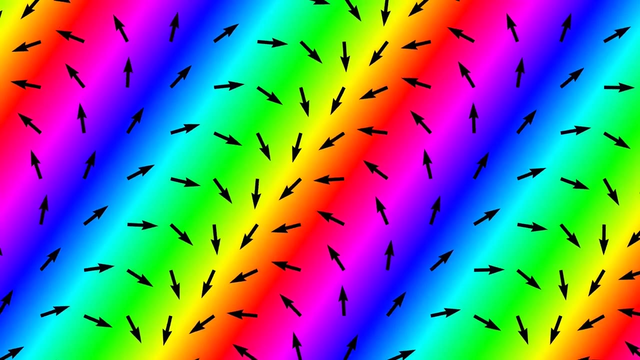 to think that the complex numbers are embedded in this two-dimensional space and that their direction is sort of pointing in a direction in that space. This is a common misconception, and I had this misconception for a while when I was learning quantum mechanics, because one of the things that confused me about complex numbers was they're two-dimensional right. 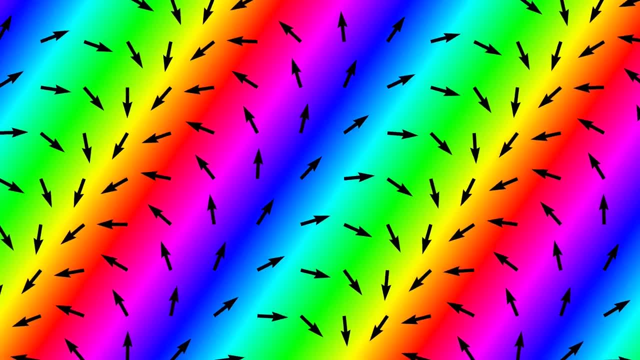 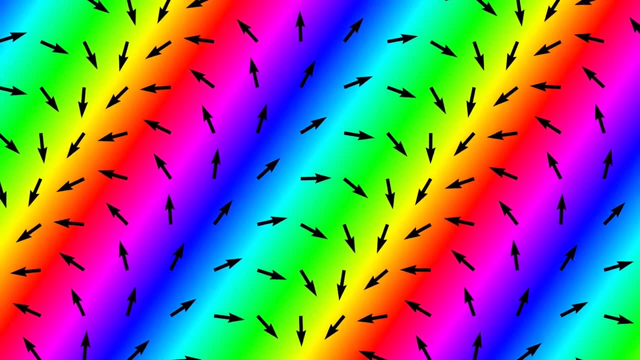 So why? I mean, if you have a three-dimensional wave function, for example, shouldn't you have like some kind of three-dimensional thing Like how do you stick a two-dimensional arrow at a point in space? How does that even make sense? But I hope that, based on everything, 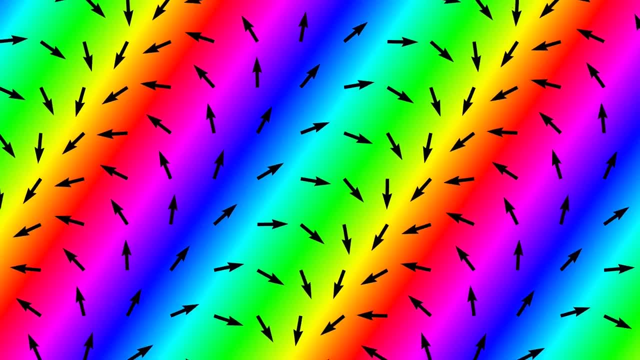 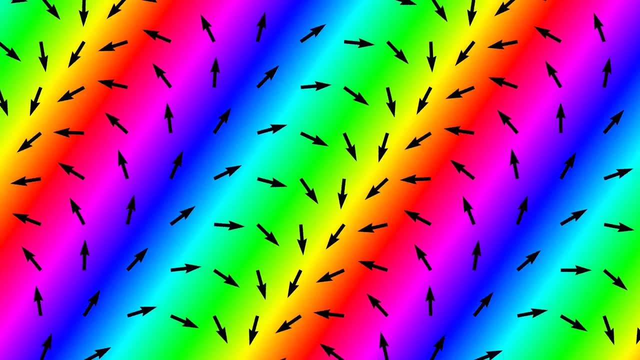 you've seen so far, you realize that the two-dimensionality of the complex numbers actually is not about any direction in physical space. The fact that the complex numbers are two-dimensional is the fact that a wave is up and down, or left and right or back and forth. It's not. 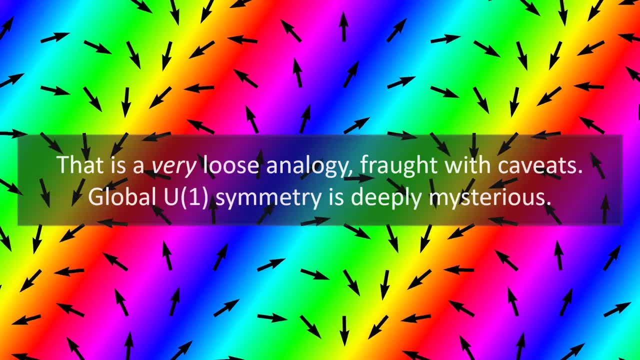 a right or left or right or left or right or right or left or right or right or left or right or right or left or left or right. It's an infinite number of dynamic and complex numbers that are all coexisting, And it tends to be the same for all of our machines. 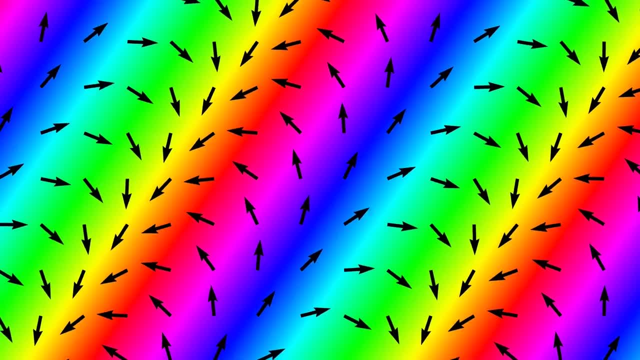 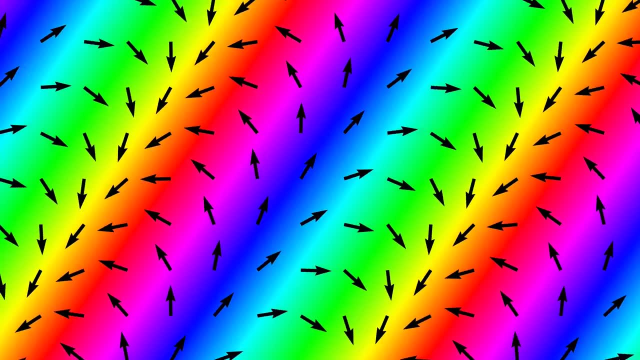 The second point I want to bring up when it comes to planewaves is that these things- you will see these all over the place- Why? A couple of reasons. One: honestly, it's kind of one of the easiest solutions to all these wave equations that you'll encounter in quantum. 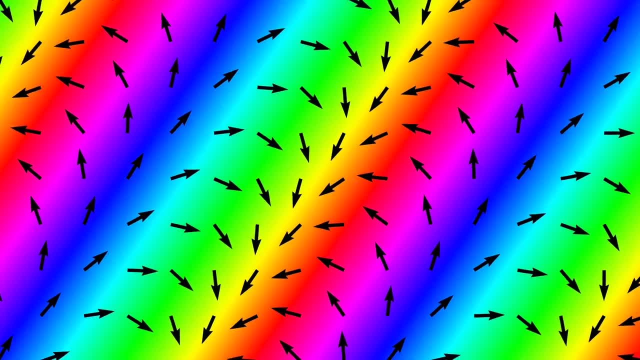 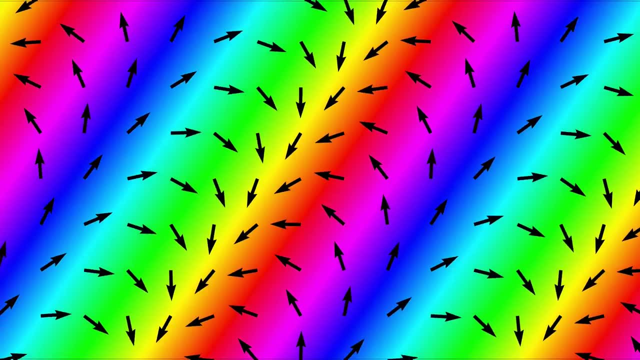 mechanics, But also it can be used as a Fourier basis to construct these more complicated wave functions, Like earlier when we looked at the square wave and you could see how you can make an arbitrary waveform by adding a bunch of waves. Well, if you take a bunch of plane waves, 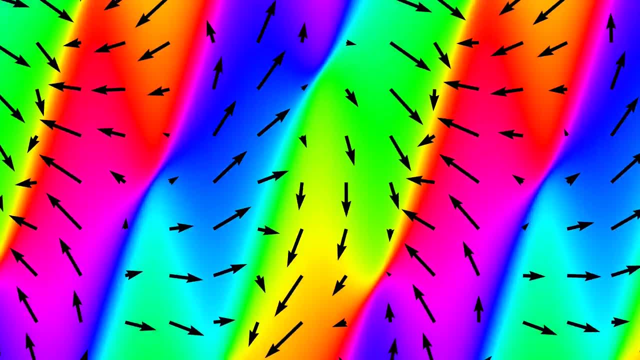 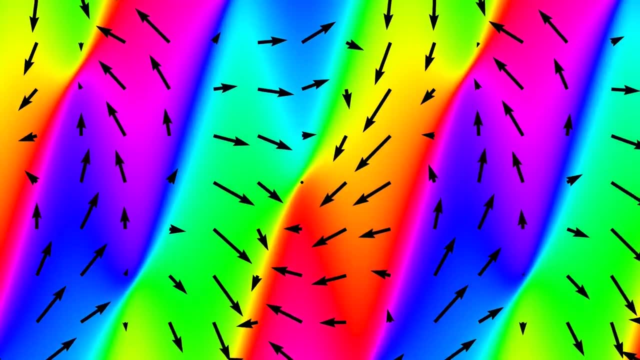 that satisfy, for example, the Schrodinger equation or the Klein-Gordon equation or the Dirac equation, although in that case you have Beispinner fields more complicated. but whatever, If you have plane waves that satisfy some differential equation and you add them, you take. 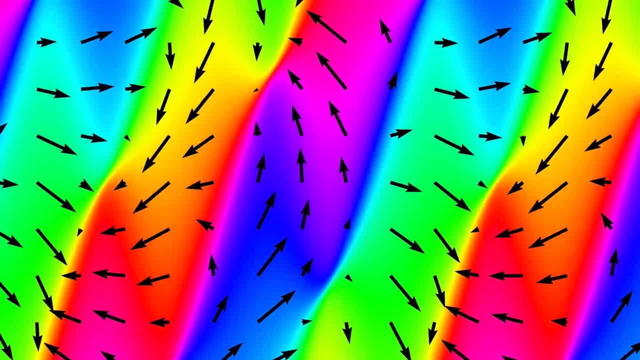 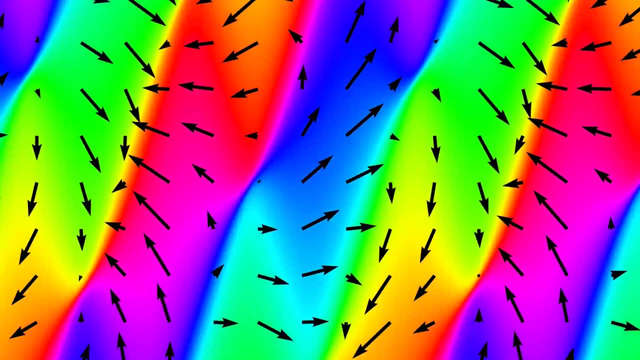 their superposition, you can create these more complicated systems that also satisfy those equations. And in fact in quantum field theory the plane waves play a essential constitutive role in the second quantization that allows you to actually make a quantum field theory. 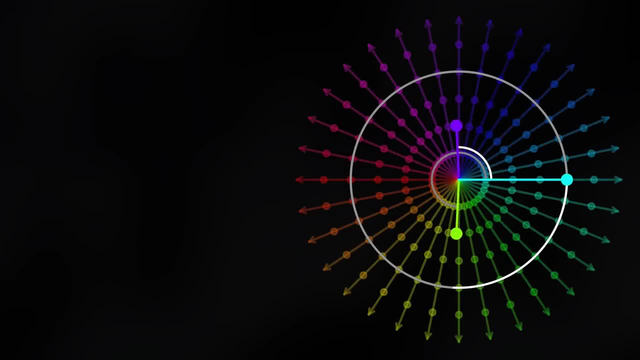 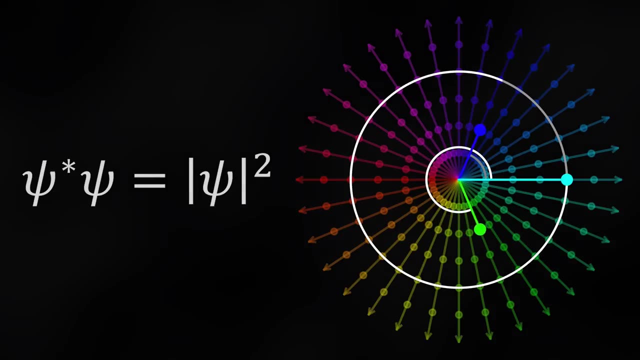 Oh, I almost forgot, but earlier, when we were looking at the complex multiplication, let's go back to that picture, except now I'm showing you something special. So these are two complex numbers that have amplitude 2 and their product has amplitude 4,. 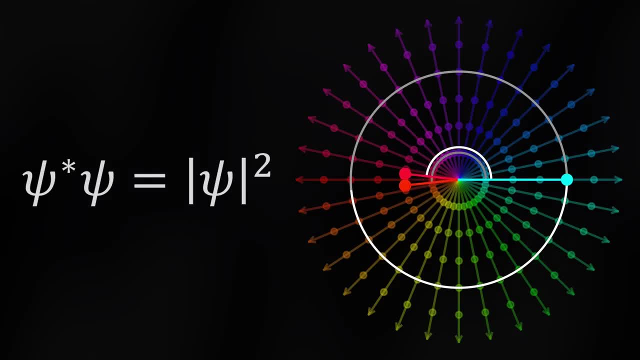 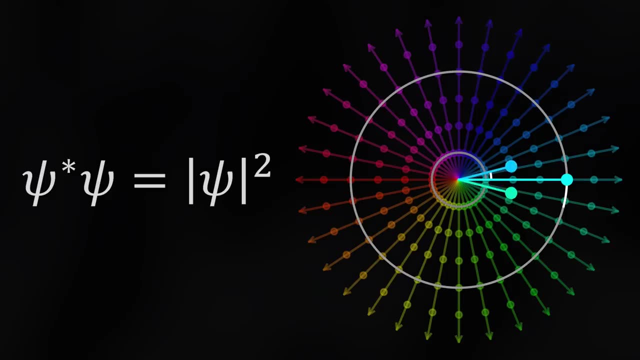 but notice, this time the two numbers are complex conjugates of one another. That means that the imaginary component has flipped sign, In other words, it's been mirrored about the real axis, And so what we're seeing here is a number times its complex conjugate. 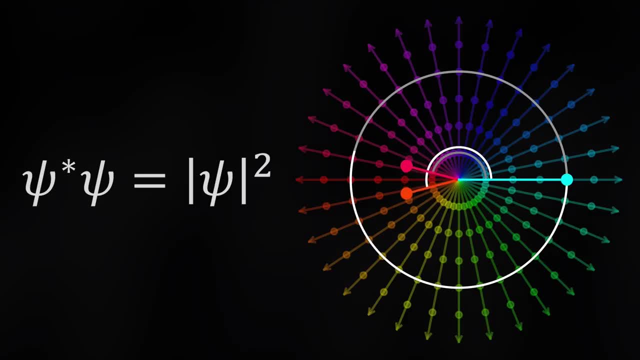 and the result is a number times its complex conjugate. And so what we're seeing here is a number times its complex conjugate, and the result is always stuck on the real number line. Why is that? Well, add the angles: A complex number. 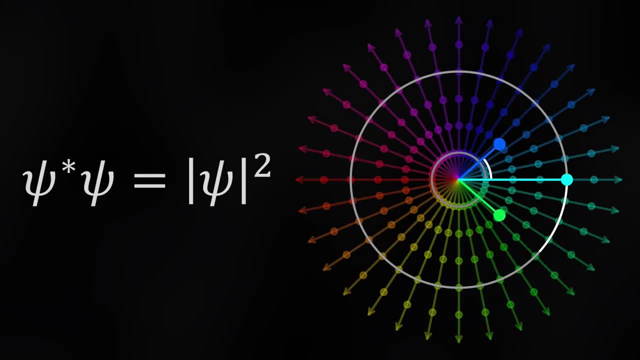 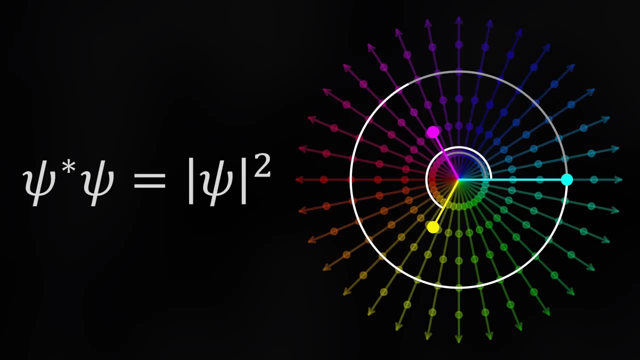 and its complex conjugate always have angles that add up such that you get back on the real axis, And for that reason you'll often see the expression psi, star, psi as a way of expressing the amplitude squared of a complex number. In quantum mechanics, psi, star and psi are very 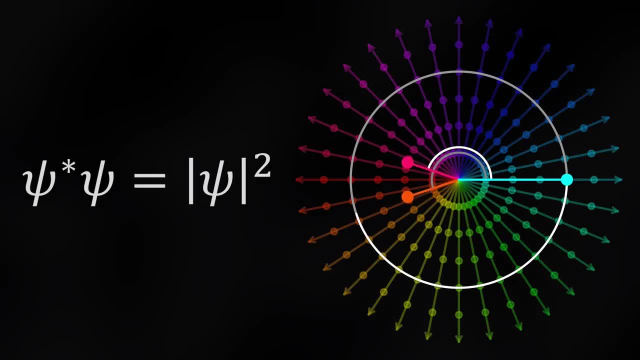 often the two slices of bread in an operator sandwich, But when you see psi star psi without any operator in between, you'll often see the expression psi star psi as a way of expressing the amplitude squared of a complex number, And so what we're seeing here is a number. 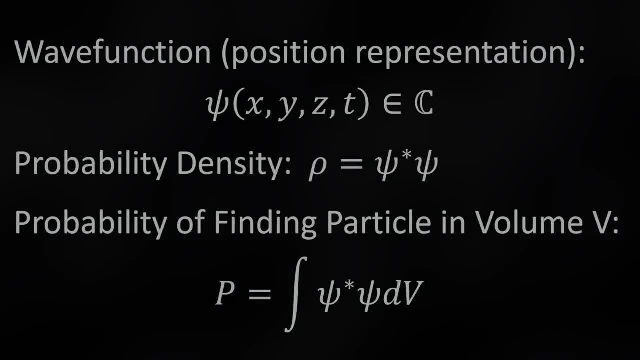 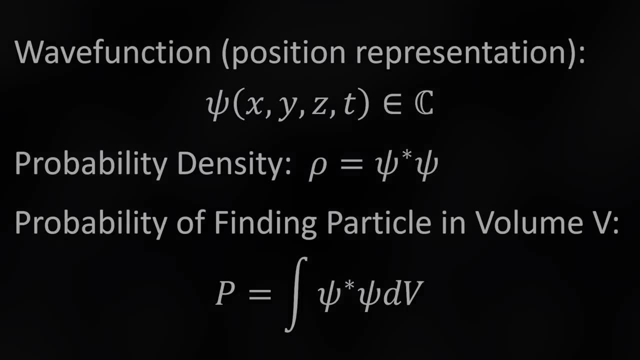 times its complex conjugate and the result is a number times its complex conjugate. and, by the way, if psi is a wave function, then psi star. psi is the probability density relating to that wave function. So if you want to find what's the probability of finding a particle, 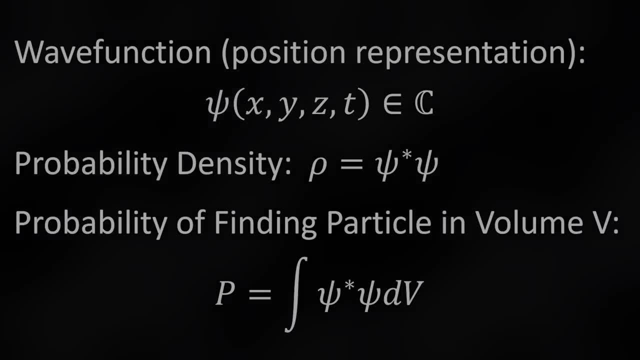 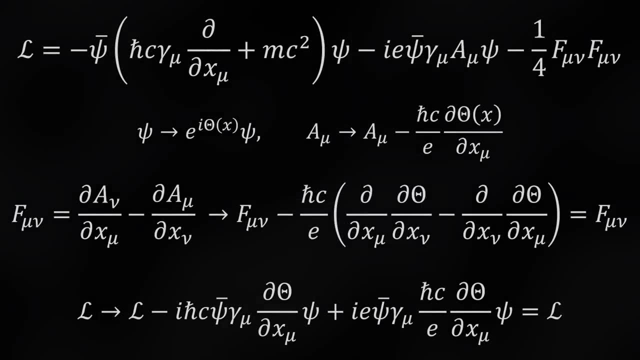 in some volume of space. you just integrate psi, star psi over that volume of space and that gives you the probability of finding the particle there. Okay, I'm going to end this video on a cliffhanger by alluding to one of my favorite ideas of. 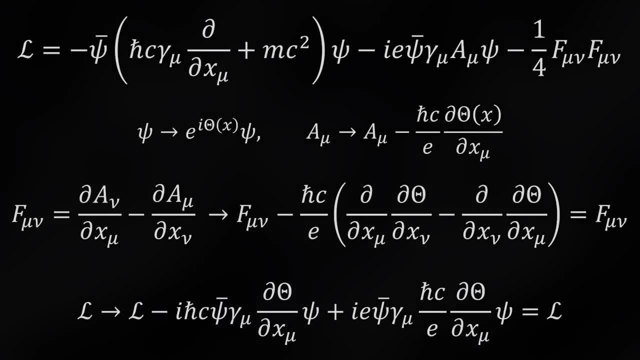 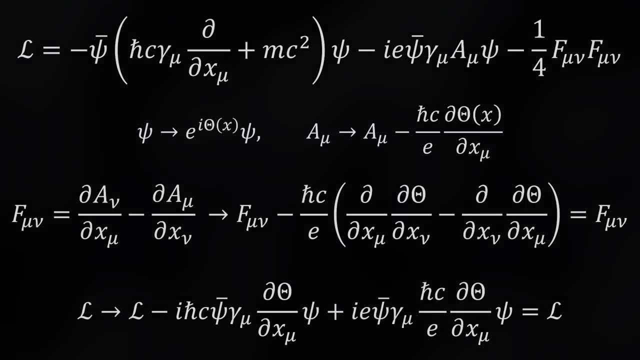 all time which is beautiful and profound and it relates to the complex numbers And that is the idea that in quantum electrodynamics a local U1 symmetry of the wave function implies electromagnetism. This is going to take a while to unpack and I am going to